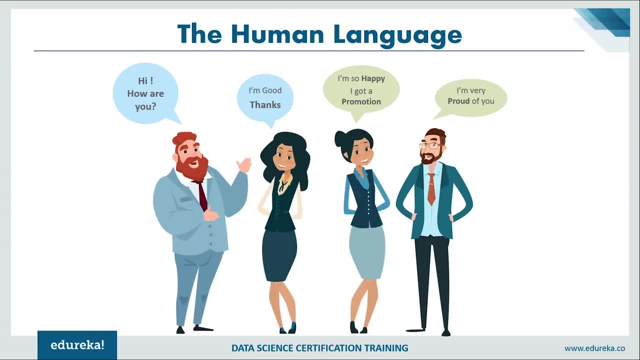 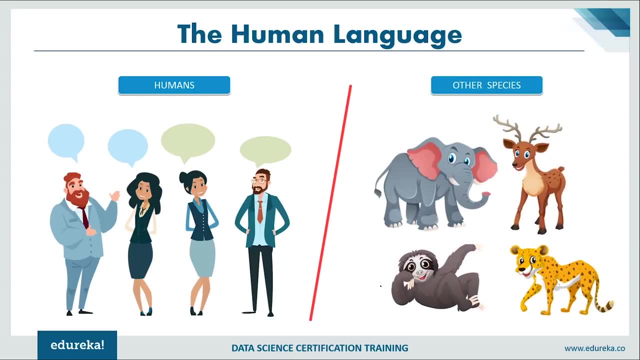 So the success of human race is because of our ability to communicate, that is, information sharing. using this ability, We have marched ahead of other animals and have become the most sophisticated creatures, and this is what differentiates us among all the other animals. We begin to look for ways to preserve our thoughts, feelings. 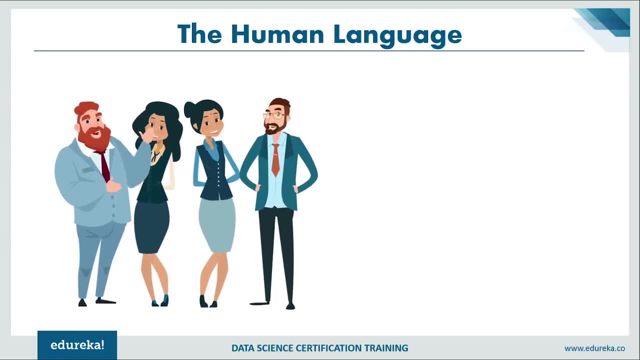 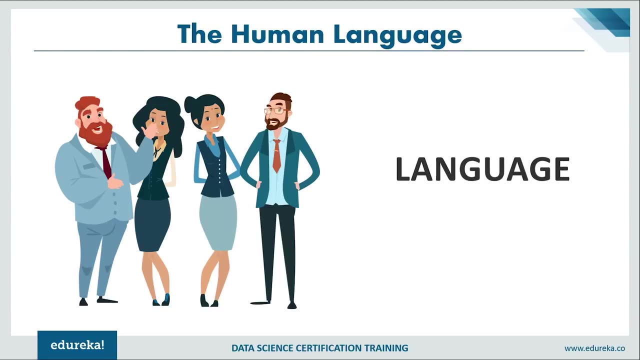 messages and other information. We started with oral communication, like other animals, but because of its a formal nature, we begin painting on walls and caves where we lived. but there was a need to standardize the drawing so that everyone could understand, and that's where the concept of developing a language came in. 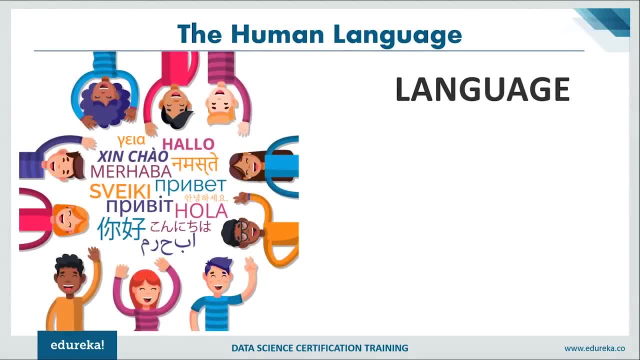 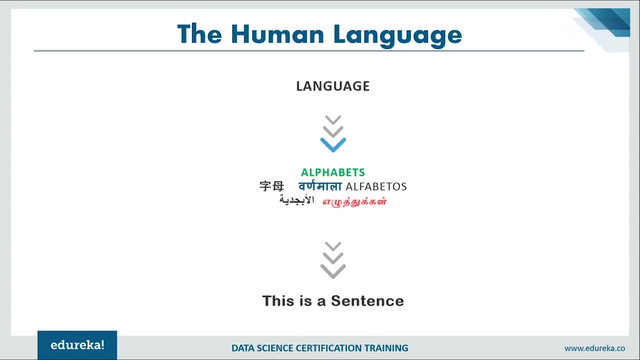 However, many standards came up, resulting in many languages, with each language having its own basic sets of alphabets, combination of alphabets which are known as words, and the combination of words which were arranged meaningfully, which became the sentence. now, each language has a set. 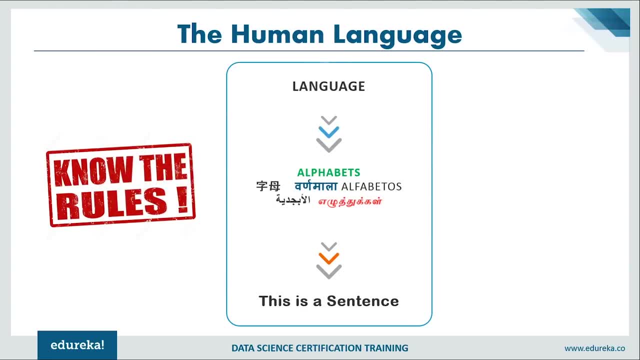 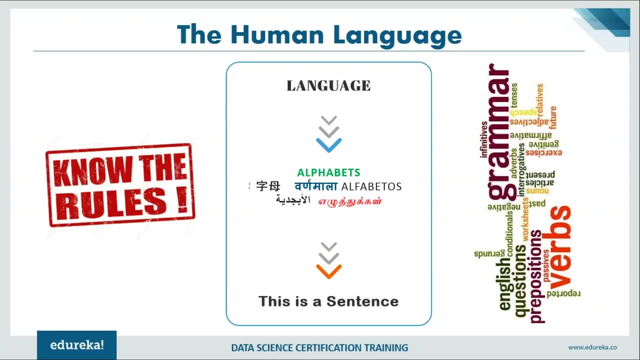 of rules based on words and are combined to form these sentences. Now, these set of rules are nothing but what we call it as grammar. Now, I'm not going to take any more time explaining you guys about grammar and all. Now coming to today's world. according to the industry estimates, 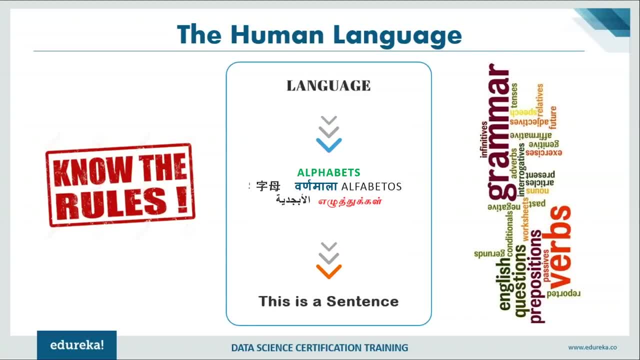 only 21% of the available data is present in the structured form. data has been generated as we speak, as we treat, as we send a message on WhatsApp, Instagram, iMessaging and various other platforms. majority of this data exists in the textual form, which is highly unstructured in nature. now, in order to produce 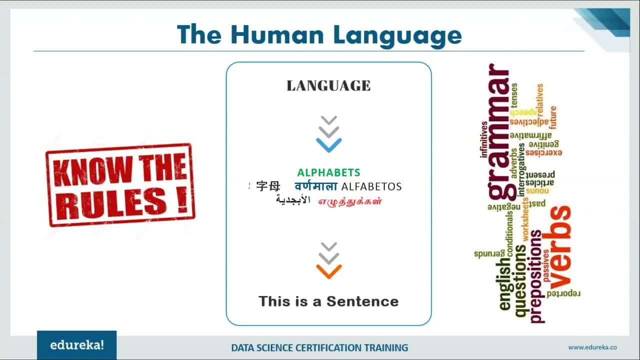 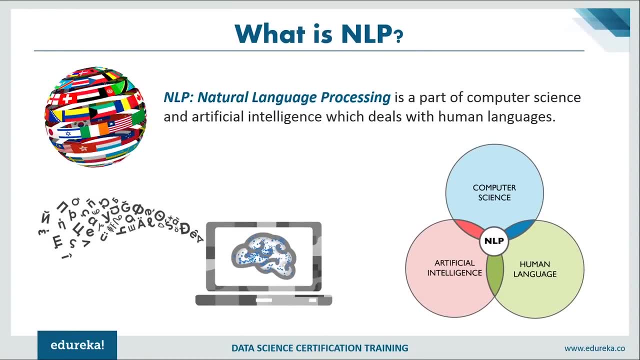 significant and actionable insights from this text data. It is important to get acquainted with the techniques and the principle of natural language Processing. so let's understand what exactly is NLP now? natural language processing- that is NLP- refers to the artificial intelligence method communicating with an intelligent system using natural 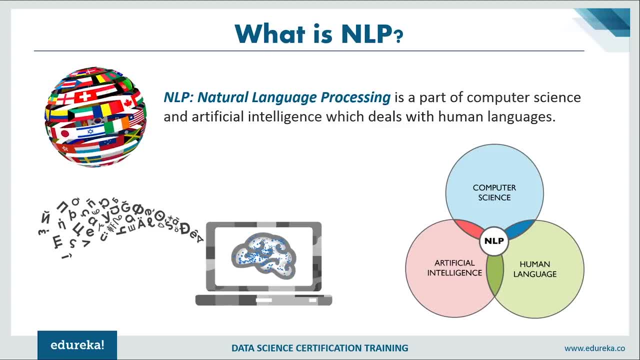 language. Now it is a part of computer science and artificial intelligence which deals with the human language. by utilizing NLP and its components, one can organize the massive chunks of text data, perform numerous automated tasks and solve a wide range of problems such as communication, summarization, machine translation. named entity. 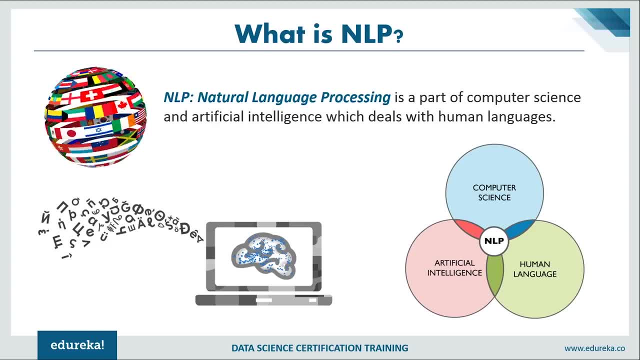 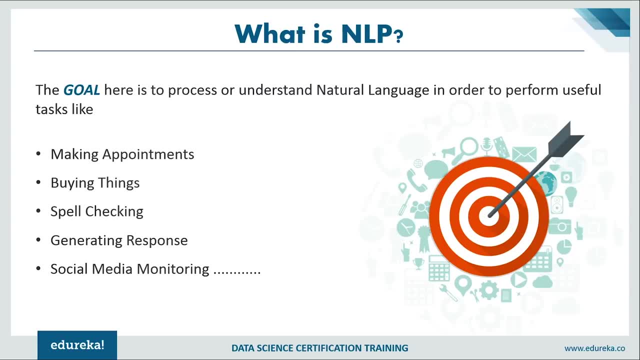 recognition, relationship extraction, sentimental analysis, speech recognition and topic segmentations. now, we'll learn about all of these later in this video. Now the goal here is to process, I'd rather say understand, the natural language in order to perform useful tasks. So these tasks includes making appointment, buying things, spell. 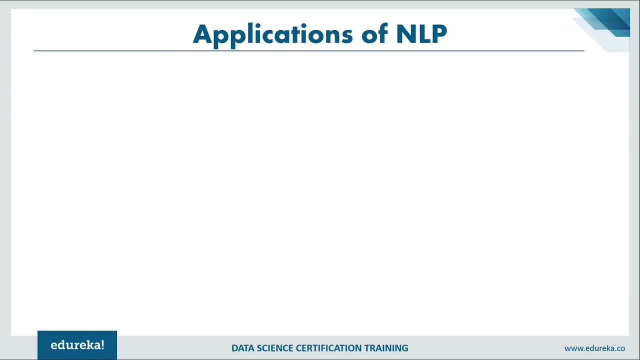 checking, generating responses and social media monitoring. Now, if you look at the various application of NLP, NLP in the industry, Firstly we have the spell checking, which is usually there in. you can find it mostly in words or the document reader, even online. 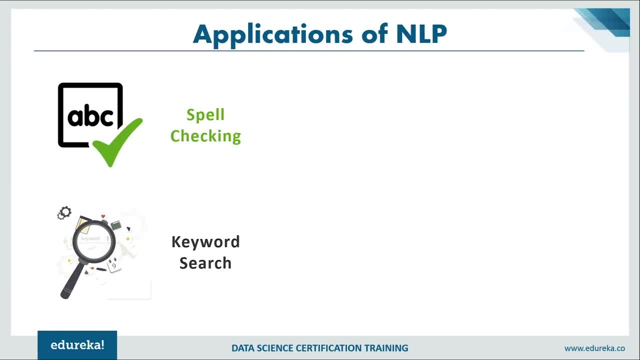 Also, you can do the spell checking now. next, we have keyword search, and it is also a field where NLP is heavily used. now, extracting information from websites or any particular document also requires the knowledge of NLP. Now, one of the coolest application of NLP is the advertisement. 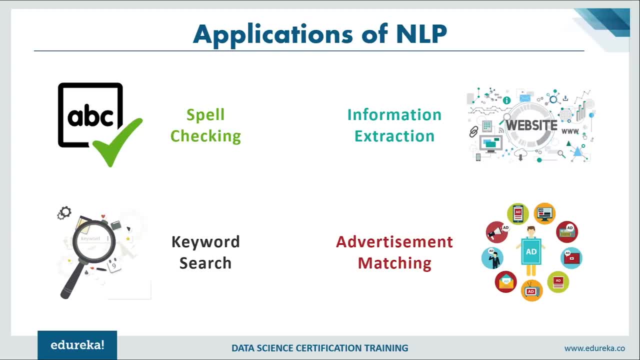 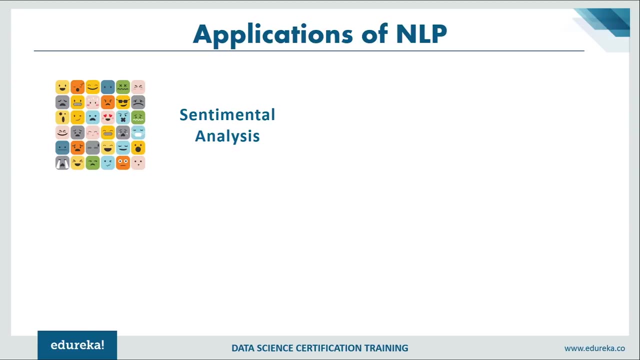 matching, which is basically recommendation of ads based on your search. What it does is analyzes the text of the data which you are already using or searched and match it with the text data of the advertisement. now, sentimental analysis is also a very major part of NLP. 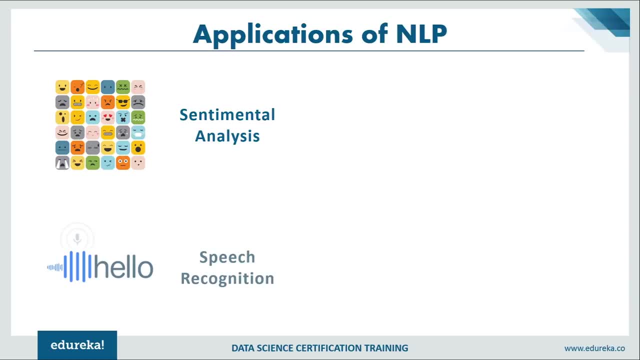 Another application is the speaker ignition. Now. here we are also talking about the voice assistants, like the Siri Google assistant, the Cortana, and we need to thank Apple for creating the first voice assistant, that is, Siri, now. next, we have the implementation of chatbots, now most. 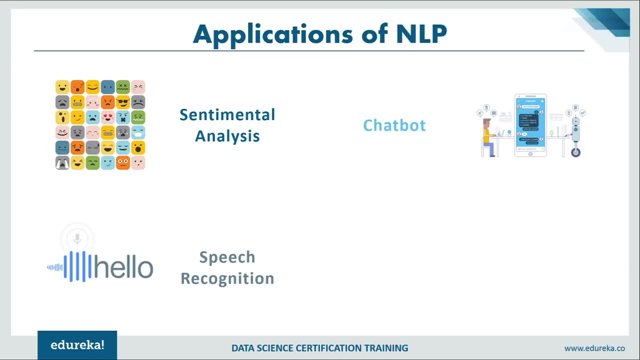 of you guys might have used the customer chat services provided in various apps. Now, most of these apps use the chatbot, which is it uses NLP to process the data which we entered and then it provides response based on an input. that is also an application of natural. 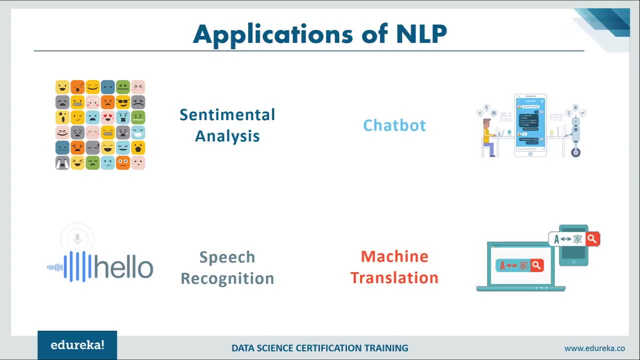 language processing. now, another application of NLP is the machine translation. Now, the most common example of it is the Google Translate, as you know, and now it uses NLP to translate the data, or I should, I'll say the text- From one language to the other, and that, too, in real time now. 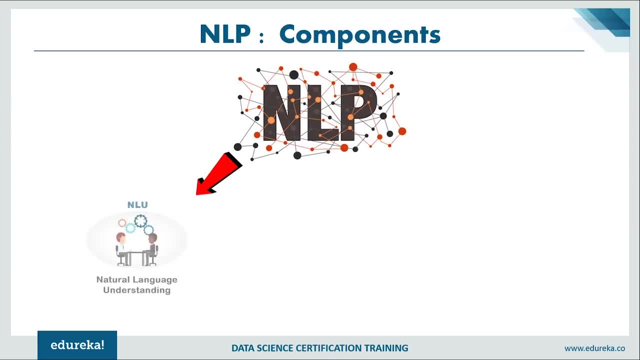 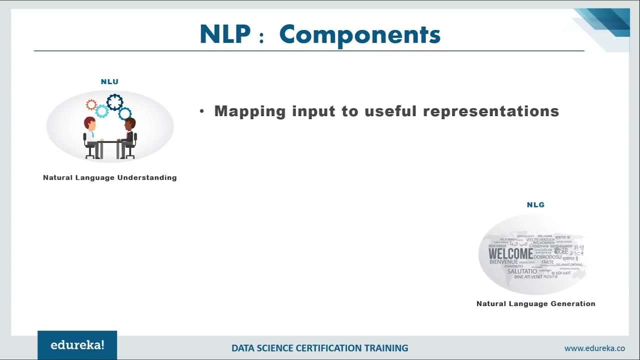 NLP consists of two components, which is the natural language understanding, referred to as NLU, and the natural language generation, which is referred to as NLG. now, understanding the natural language involves mapping the giving input in natural language into useful representation and analyzing different aspects of the language. now, natural language generation is 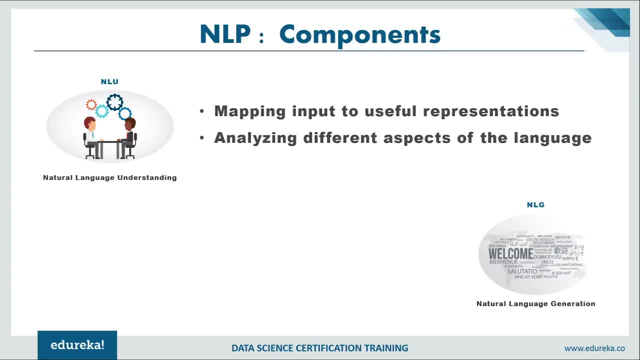 the process of producing meaningful phrases And sentences in the form of natural language from some internal representation. now it involves text planning, which includes retrieving the relevant contents from the knowledge base. It involves sentence planning, which includes choosing require words from meaningful phrases, setting tone of the sentences. 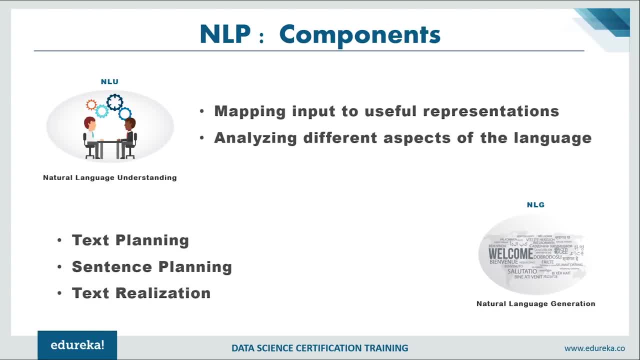 and finally we have text realization. It is mapping sentence plan into the sentence structure. now we'll learn about this later in this video, and usually natural language understanding, which is NLU, is much, much harder than NLG. now you might be thinking that even a small child- 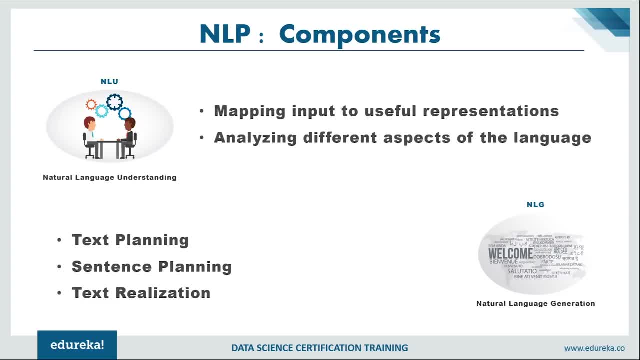 can understand a language. So how come it is so easy for human beings are so difficult for the computer to process it? So let's understand what are the difficulties a machine faces while understanding a language. So in natural language understanding there are certain ambiguities. 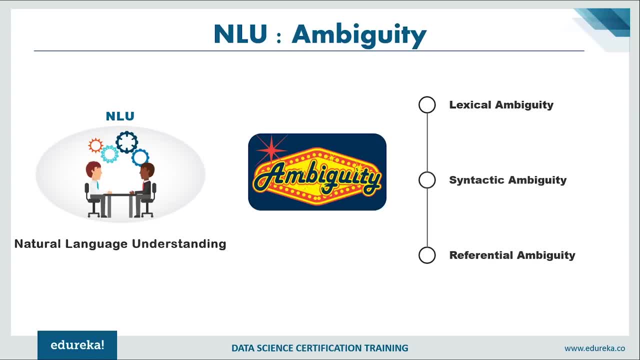 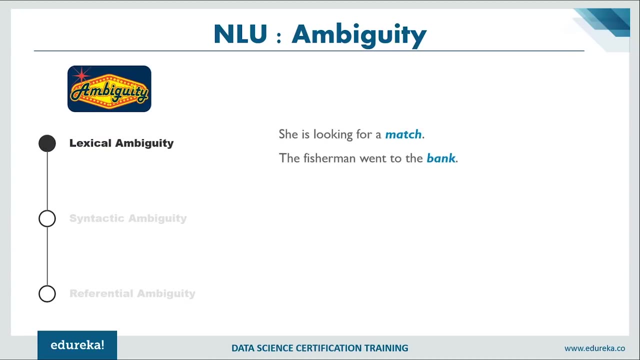 which are the lexical ambiguities, syntactical ambiguity and the referential ambiguity. now, understanding a new language is very hard. taking our English into consideration, There are a lot of ambiguity, and that to in different levels. now, starting with lexical ambiguity. lexical ambiguity is the presence of two or more possible meanings within a 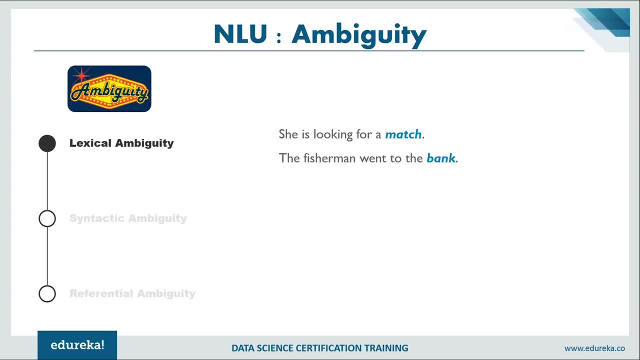 single word. It is also called semantic ambiguity. For example, let's consider the following sentences and let's focus on the italicized world. Now She is looking for a match. Now, what do you infer here from the match world? Is she looking for a match that is head to end match, or is 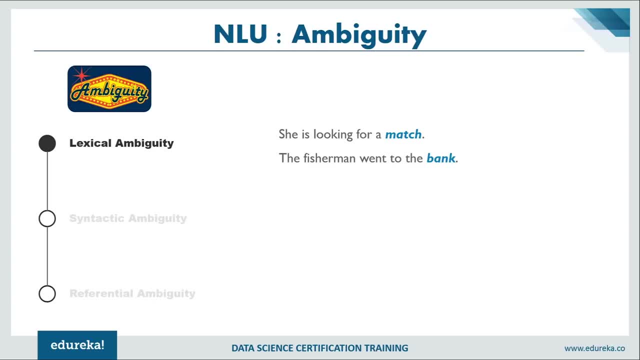 you looking for Match? as in a partner, the fishermen went to a bank. Is it the bank where we withdraw our money or is it the bank where he rose his boat or he catches the fishes now? syntactical ambiguity. in English grammar, This ambiguity is the presence of two or more possible meanings. 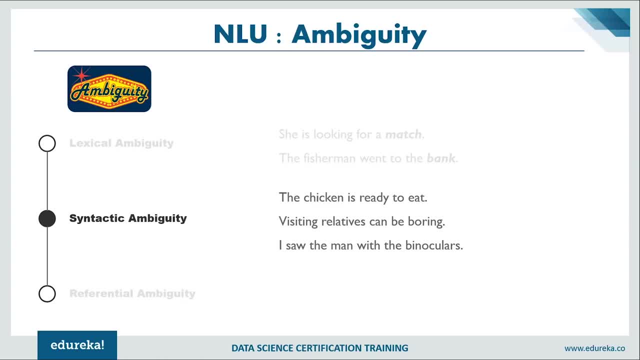 within a single sentence or a sequence of words. It is also called structure ambiguity or grammatical ambiguity. Now Let's have a look at these sentences. The chicken is ready to eat. So is the chicken ready to eat something, or is the chicken? 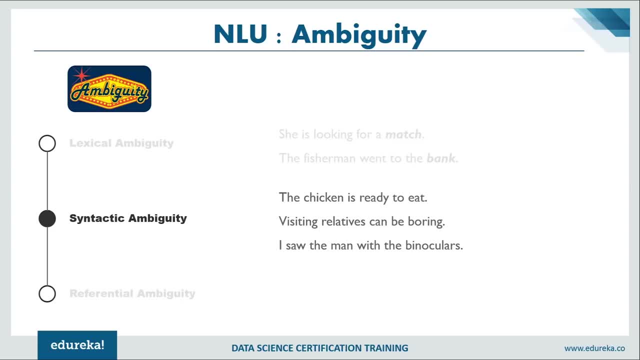 ready for us to eat. So this is a kind of syntactical ambiguity which is often very hard to info for a new person, or I'd rather say a computer, because it means the meaning of the sentence is different for the different tones or in different aspects. 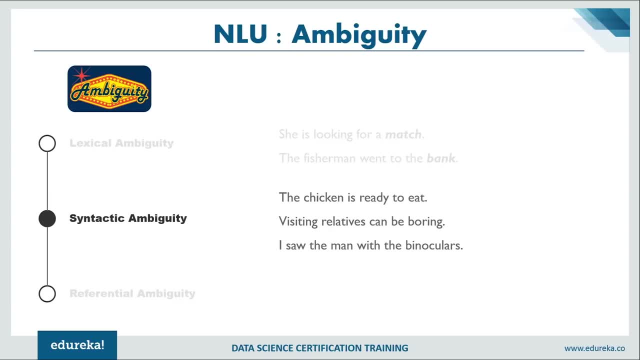 So, for example, if I look at the last statement, I saw the man with the binoculars. So do I have a binocular, or the man has a binocular? It might be possible that you might be thinking that I saw the man with binoculars means that I have the binoculars, but somewhere. 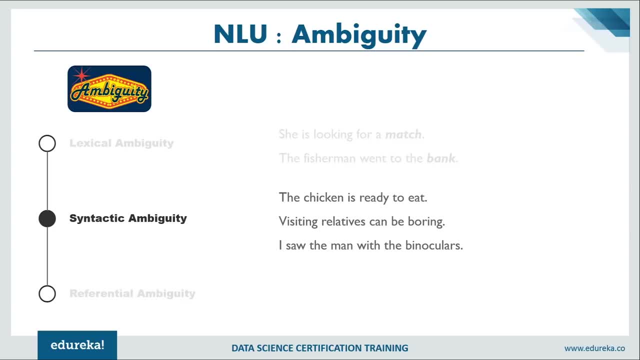 some people might think that the guy which I am seeing has the binoculars rather than me. So that is syntactical ambiguity. now coming to the third ambiguity, which is the referential ambiguity. Now, this ambiguity arises when we refer to something using pronouns. 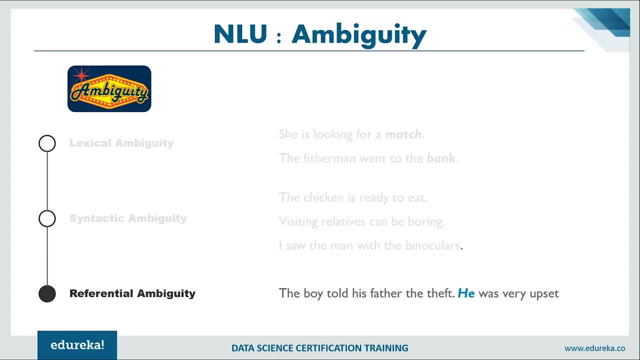 Now the boy told his father the theft. He was very upset. now, when we talk about he was Very upset, If you focus on the italicized word he, does this mean that the boy was upset or the thief was upset or the father was? 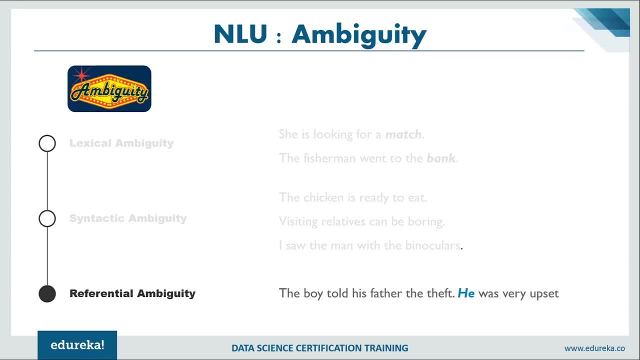 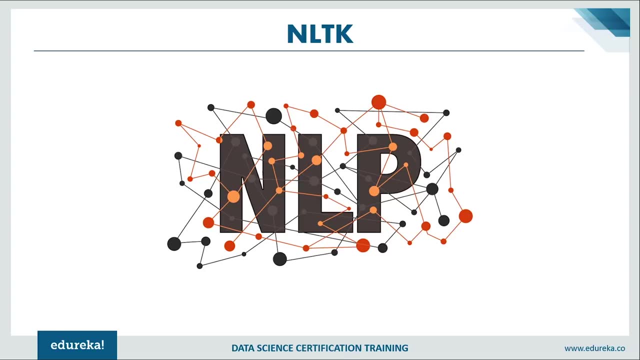 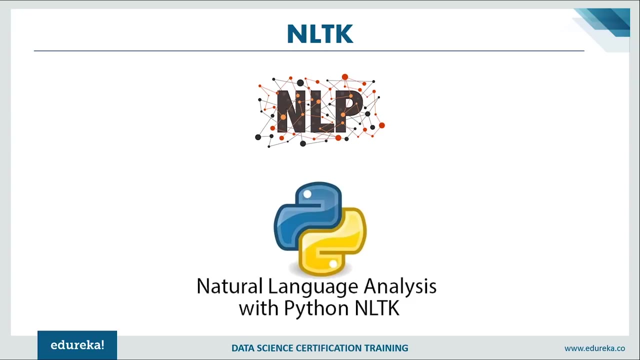 upset. Nobody knows, this is referential ambiguity. now coming back to NLP, for using NLP onto our system or doing any natural language processing, We need to install the NLTK library. that is the natural language toolkit. So NLTK is a leading platform for building Python programs to 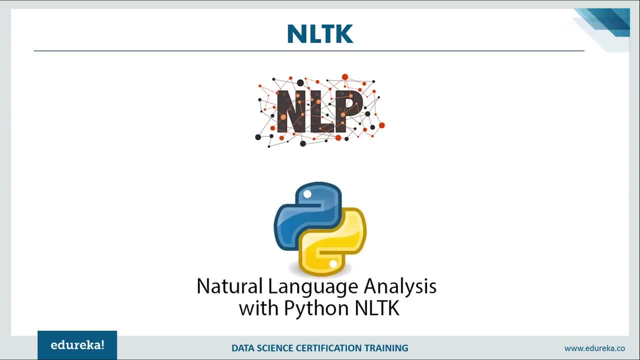 work With human language data. It provides easy to use interfaces to 50 corpora and lexical resources such as word net, along with the suit of text processing libraries for classification, tokenization, stemming, tagging and much more. Now let me show you how you can download NLTK. 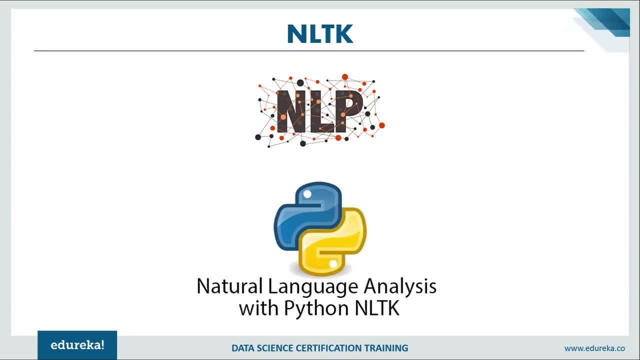 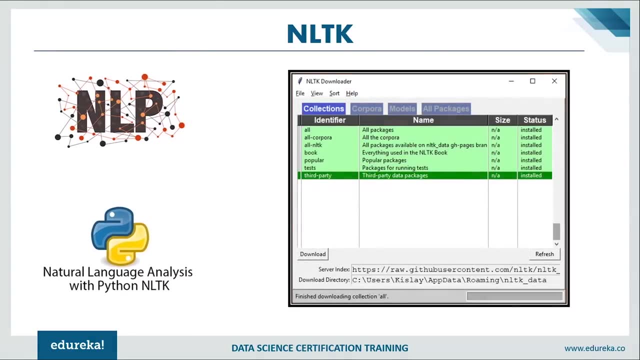 Now, in order to download NLTK, just go to your python shell and just type in the word NLTK, dot download, using the parenthesis, and then you will get this type of Window pop-up, which is the NLTK downloader. You just need to select all option and click on the download. 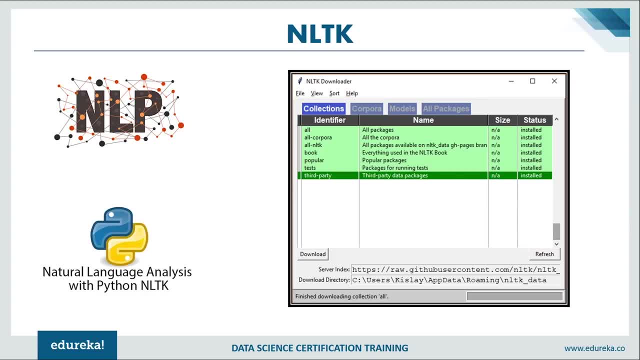 button and it will download all the corpora and the text It has, all the packages It has, into one single place and you can choose the directory where you want to install it. It's better if you download it in your python directory only it will be easier for you to access all the files and all 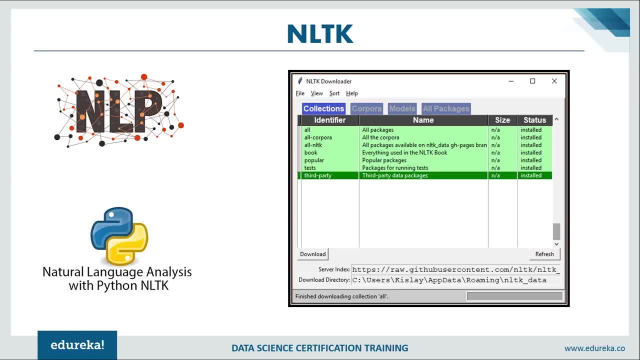 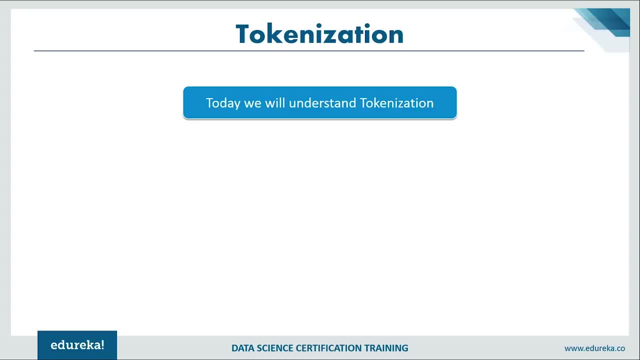 the texts which it has to offer. now, when we process text, There are a few terminologies which we need to understand. So the first terminology here we are talking about is tokenization, So it is a process of breaking up strings into tokens which, in 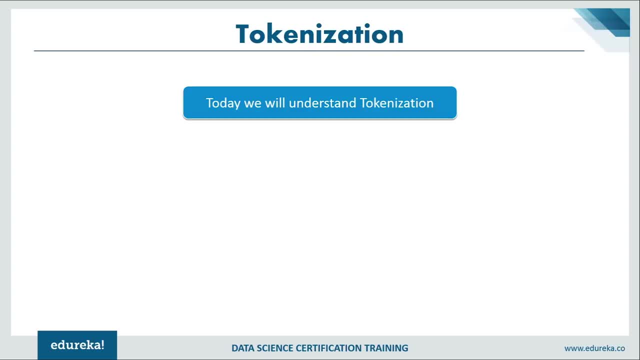 turn are small structures or units that can be used for tokenization. right involves three steps: breaking a complex sentence into words, understanding the importance of each of the words with respect to the sentence and produce a structural description on an input sentence. So if we take the sentence today, will understand tokenization. 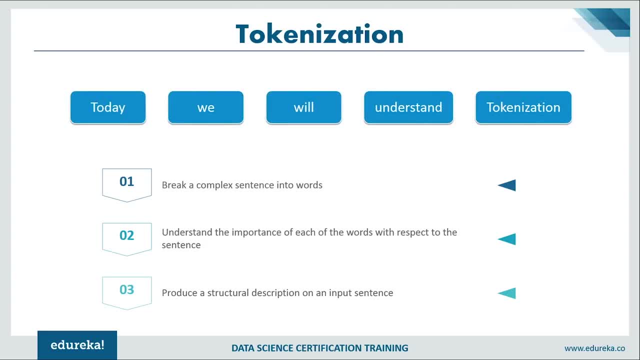 So, as you can see, we have five tokens. The first one: today we will understand tokenization. So all of these words in computer terms are known as tokens and this is what is referred to as tokenization. So let me show you, guys, how you can implement tokenization. 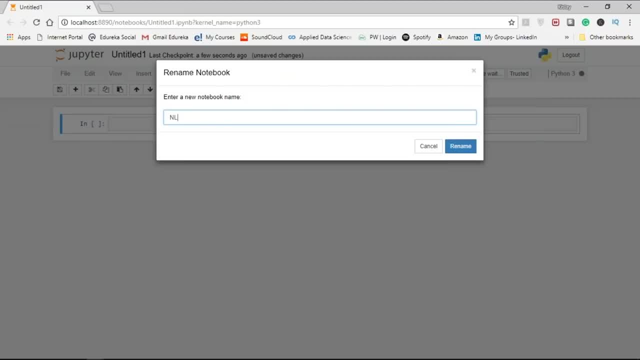 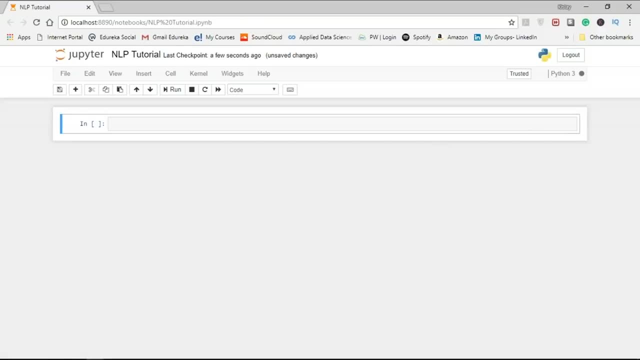 using the NLTK library. So here I'm using Jupiter notebook. You are free to use any sort of ID. also, my personal preference is Jupiter notebook. So first of all let's import the OS, The NLTK library which we have download, and the NLTK corpus. 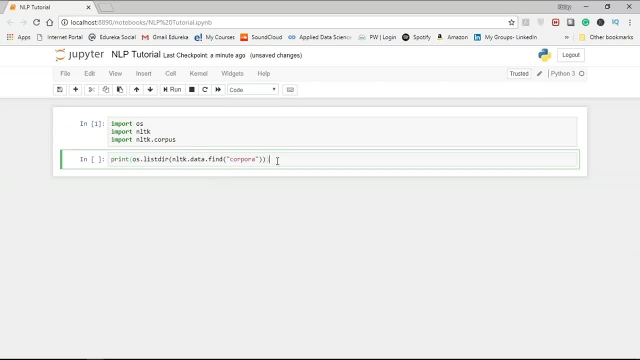 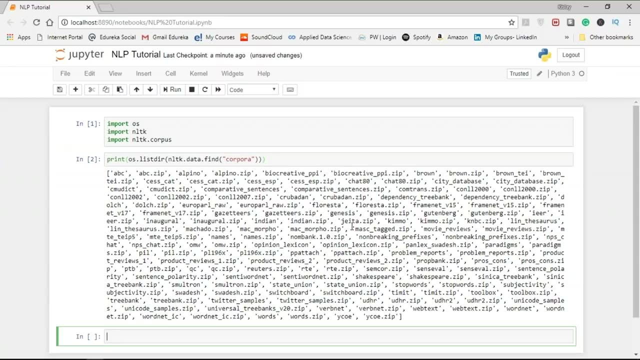 Now let's have a look at the corpora, which is being provided by the NLTK. that is the whole data. So, as you can see, we have so many files and all of these files have different functionalities. Some have textual data, some have different functions associated. 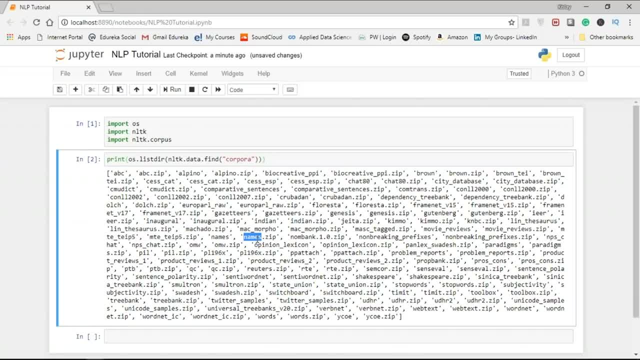 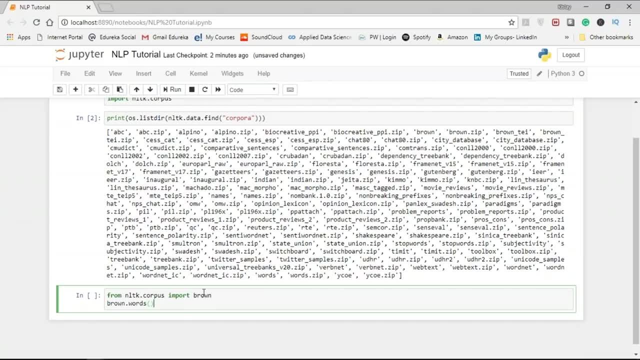 with it We have stop was, as you can see here, the State Union names. We had to just sample data. We have different kind of data and different kind of functions, So let's take the brown into consideration. as you can see here, We have brown and brown zip. 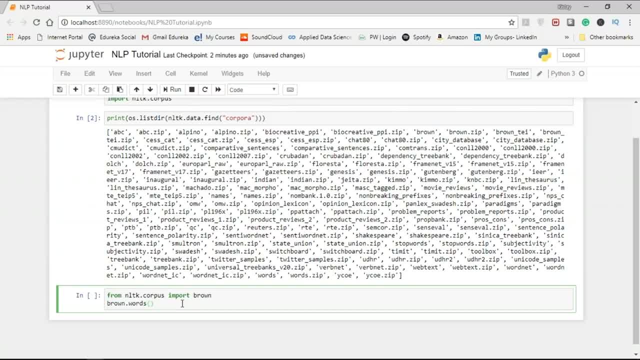 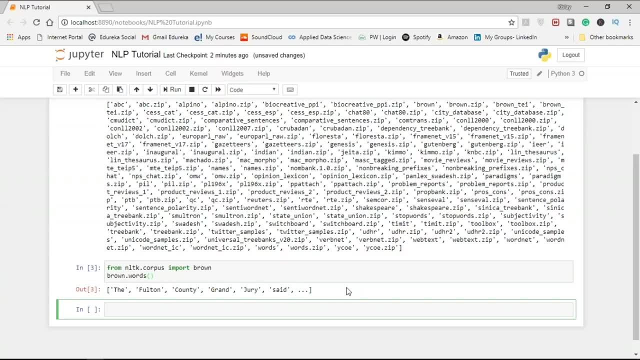 So first we all we need to do is import the brown, and then let's have a look at the words which I present in the brown. you see, we have the Fluton country Grand Jury said: and it's going on and on. Now let's have a look at the different Gutenberg fields. 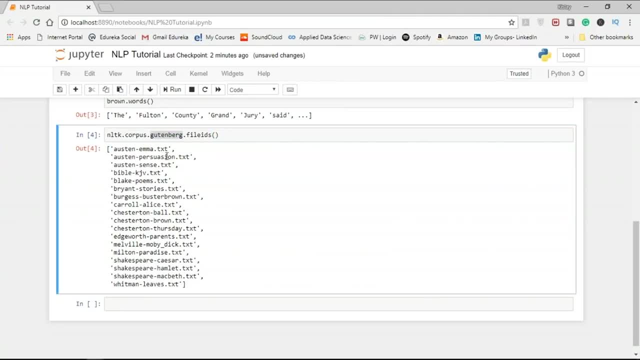 So, as you can see, under Gutenberg file, we have Austin MR text, We have the Bible text, We have the Blake poems, The Carol Alice text. Yeah, the edgeworth parents dot txt. Shakespeare's We have. we have this Shakespeare. 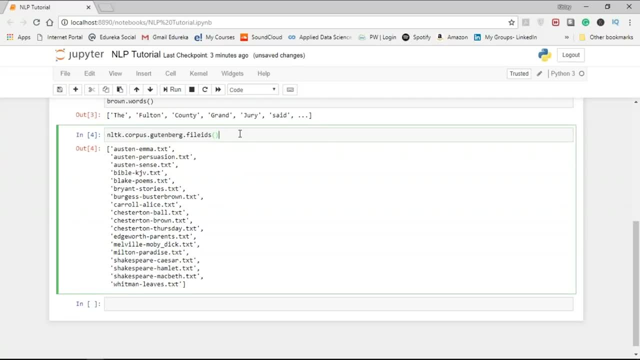 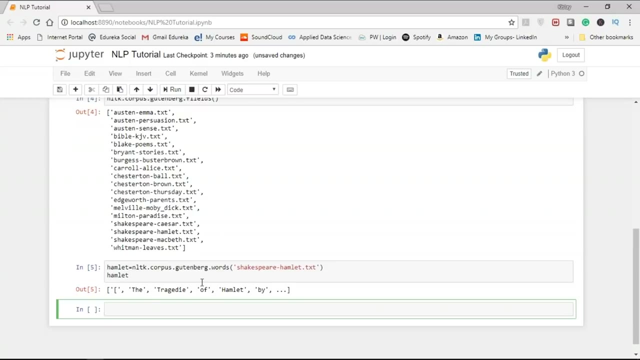 We have the Whitman leaves. So NLTK is a very big directory and a very big library to download. You might need a couple of minutes to download this library. So let's take the Shakespeare Hamlet dot txt. And if you look at the words which are inside this Hamlet file, 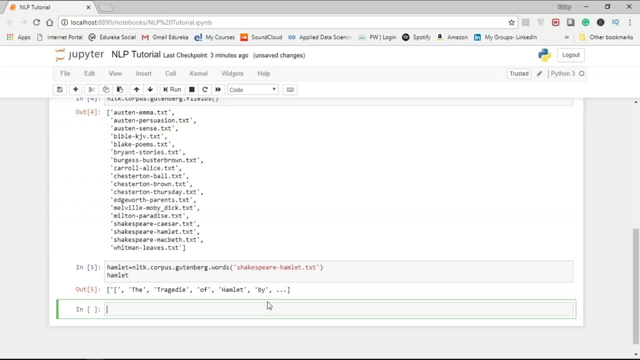 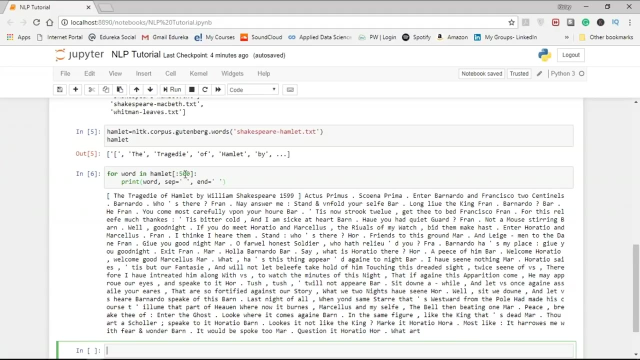 we see it starts with the tragedy of Hamlet by, and it goes on and on. So if we have a look at the first 500 words of this textual paragraph, or what we say, the text will file. So I'm using here for word in Hamlet and I'm using the colon. 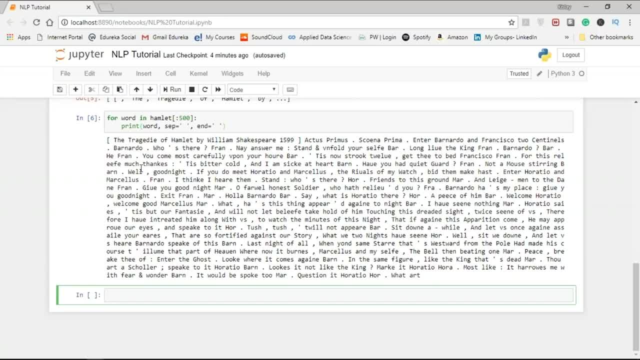 and 500. that is the end point. So, as you can see, it starts as the tragedy of Hamlet by William Shakespeare, 1599 Actus Primus Skona Prima, and it goes on and on. so for natural language processing you can use either. 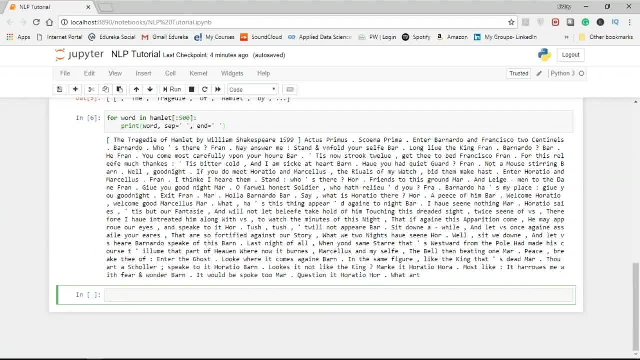 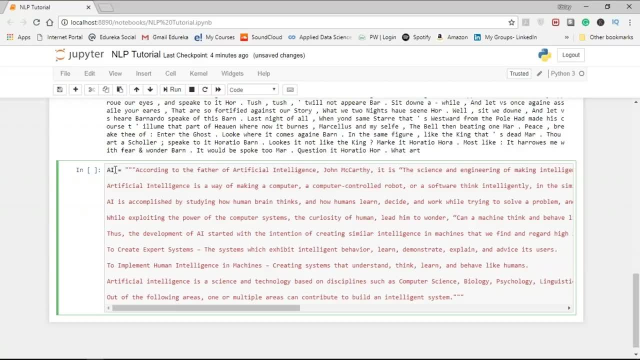 of the text which is provided here for understanding, Or you can create your own words. So, for example, here I have defined a paragraph based on artificial intelligence. Okay, so it goes on like: according to the father of artificial intelligence, John McCartney, It is the science of engineering, and so on and on. 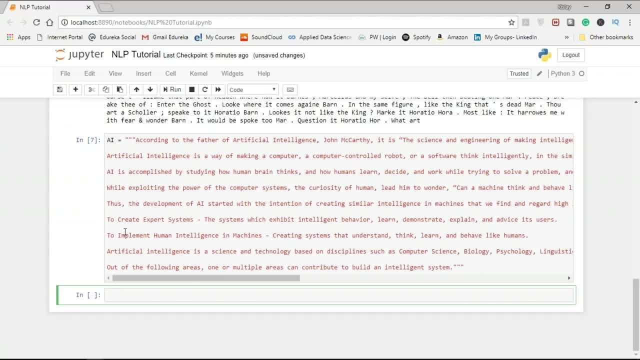 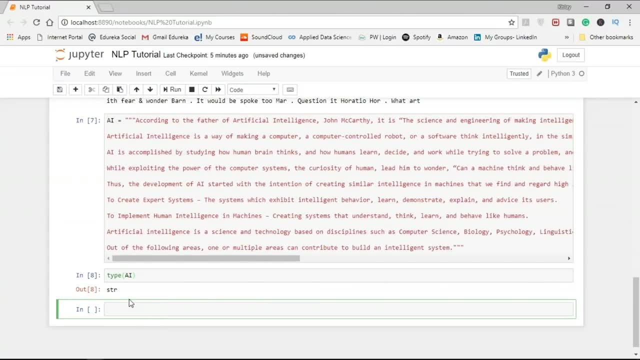 So let us first define this string. Okay, AI. now, why I'm thinking a string is because it is easy to show you guys how to work on a string. So if we do the type AI, you can see it is STR with a string now under NLTK. 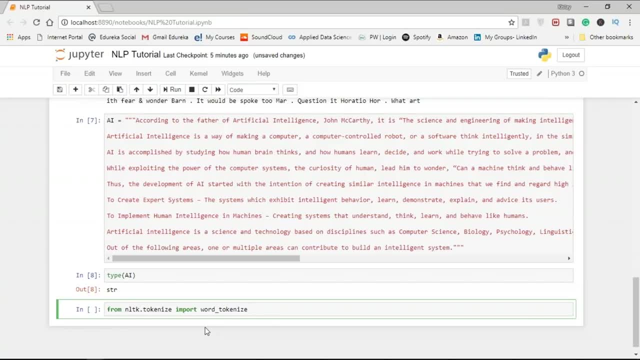 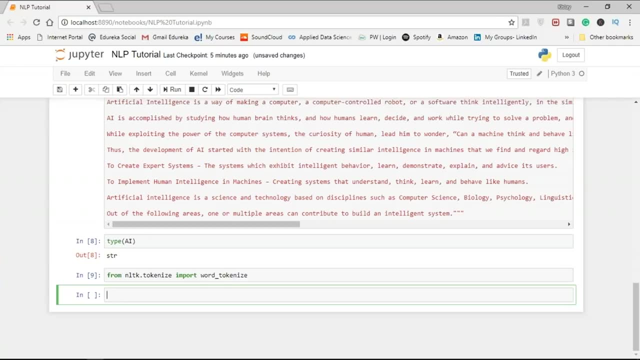 We have the NLTK tokenize and we are going to import the word tokenize right as a function will understand how it works. Now we will run the word underscore tokenize function or the paragraph and assign it a name. Let's assign it as AI underscore tokens. 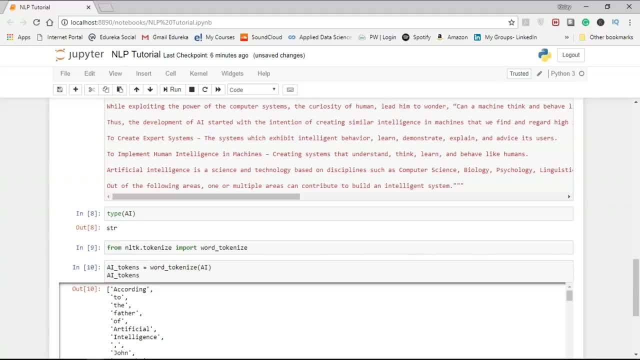 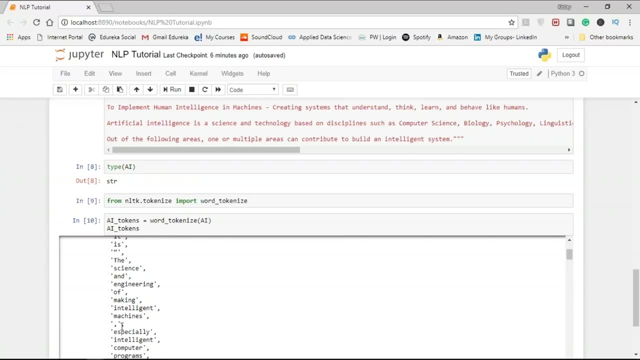 So now, if we'll have a look at the end of school tokens, you can see it has divided the whole AI paragraph which we gave into tokens. So, as you can see, it has taken a comma also into consideration, the hyphen also, and it goes on and on. now let's have a look. 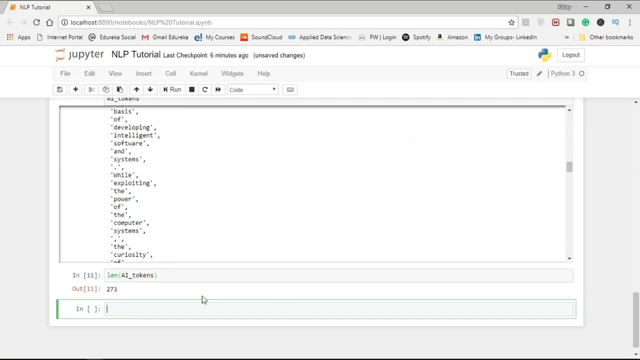 at the number of tokens where we have here. So for that we are going to use the length function. So, as you can see, we have 273 tokens now from NLTK. We have a probability function which is the frequency distinct. So I'll show you what it does. 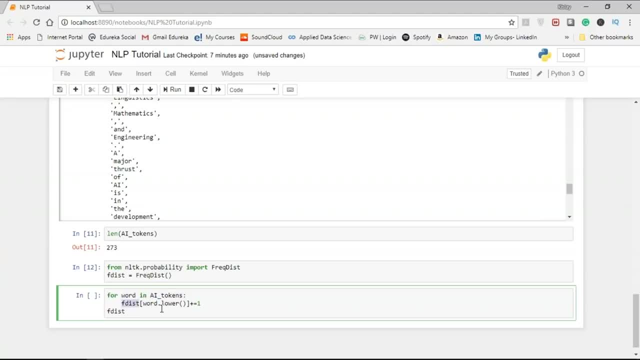 So for a word in a underscore tokens F test, and we are going to convert it to lower case so as to avoid the probability Of considering a word with uppercase and lowercase as different, and then we are going to assign it a number. This is basically a word count program and this is being 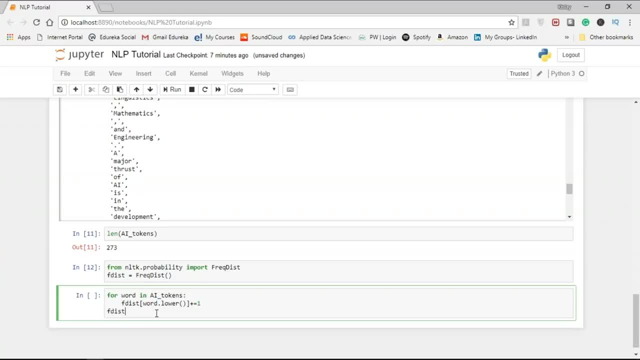 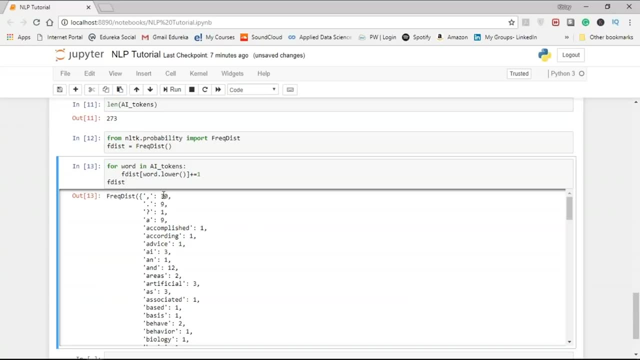 implemented using the frequency distinct function, which is already present in the NLTK library. So let's see what's the output of this one. So, as you can see it, comma has appeared 30 times, full stop has appeared nine times, question mark one, and so on and on, like. 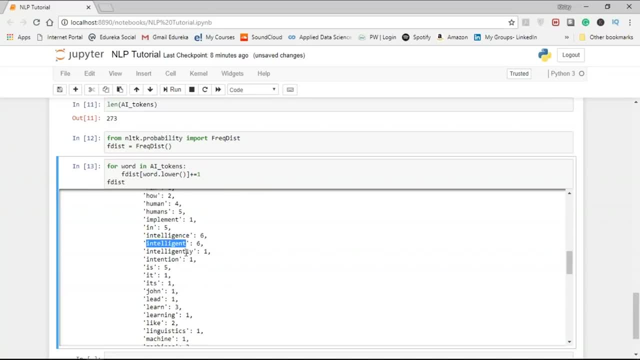 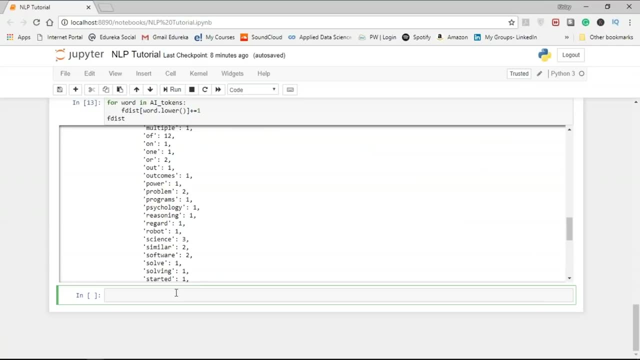 you see, intelligence has appeared six time intelligent, six time intelligent. It has appeared one time. Now, suppose, if you want to know the frequency of any particular word here. So for that we are going to use the function F test. that is the distinct frequency. 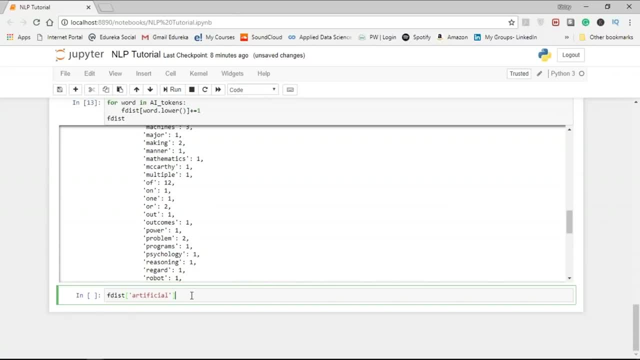 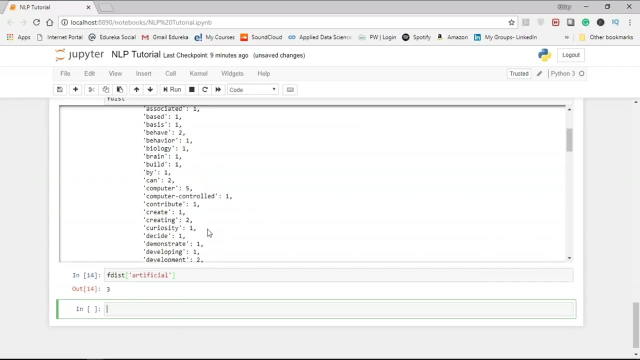 So we are going to use that function over the particular word. So, for example, let's say I want to know the frequency of artificial here. So as you can see, it is three times and if we check it in the database you can see it is artificial. 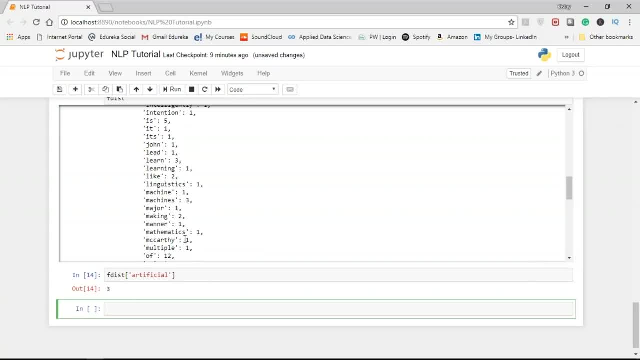 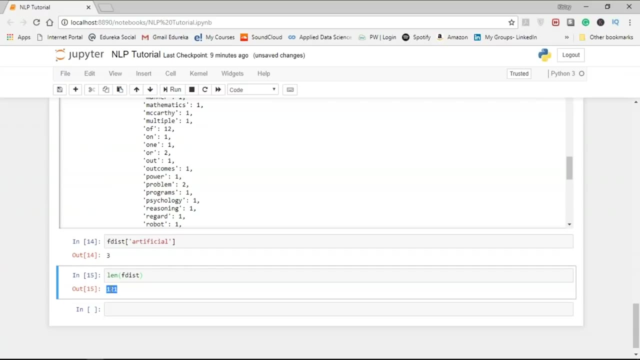 It has given us three. now, if you want to have an look at the number of distinct words here, All we need to do is pass on the F test function to the length function, So you can see it's 121.. So earlier we had 273 tokens and now from that we have 121. 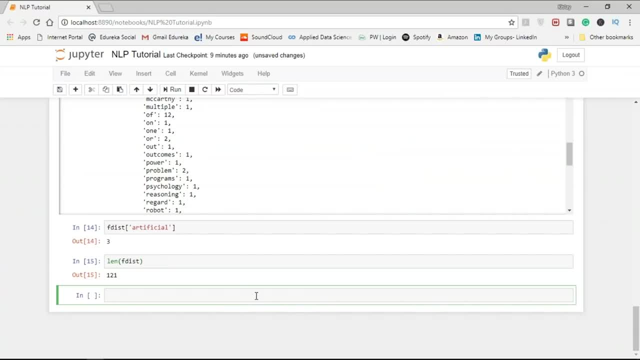 distinct tokens. Now suppose if we were to select the top 10 tokens with the highest frequency. for that I am assigning a new F, this underscore top 10- and I'm using the most underscore common function here and passing 10. that is the number of items I want. 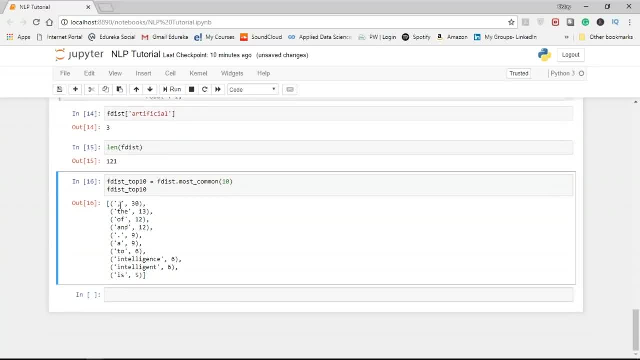 So let's see the output. So, as you can see, as I mentioned earlier, comma appears 30 times- that is the highest frequency of any word- and is appears five times. So these are the top 10 words which are the most reoccurring. 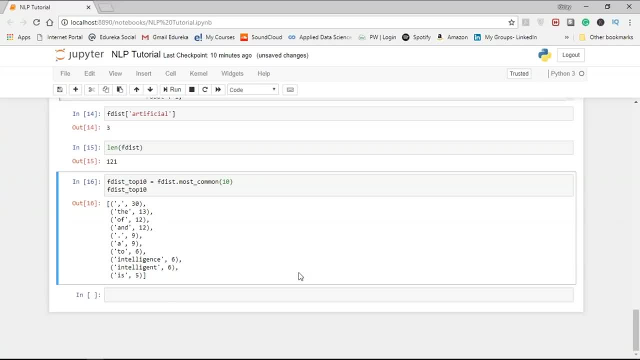 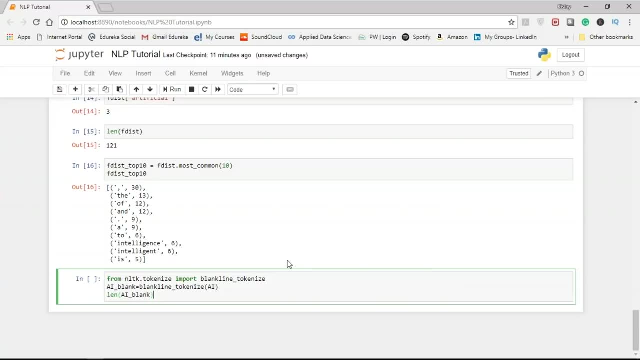 words in the given paragraph or the given sentence. Now let's use the blank line tokenizer over the same string to tokenize a paragraph with respect to a blank string. So, as you can see, we are importing the blank line in this code tokenize earlier. 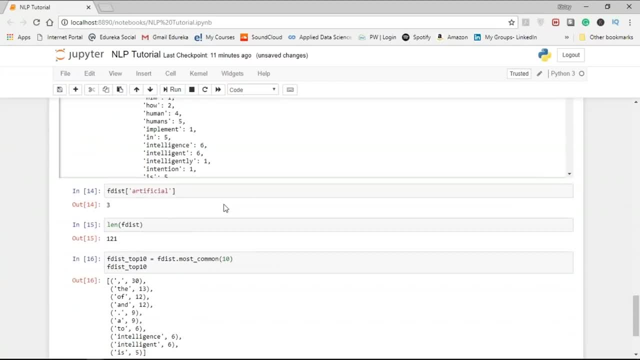 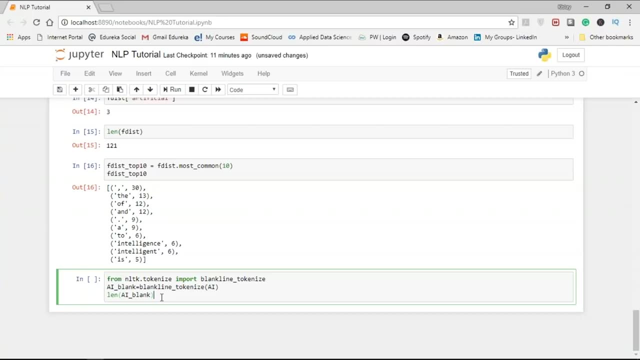 What we did was import the word underscore tokenize, and now we are using the blank line and because tokenize, and again we are passing the same AI paragraph which I gave earlier, and then we are checking the length of the a underscore blank. So, as you can see, it provides us the output 9.. 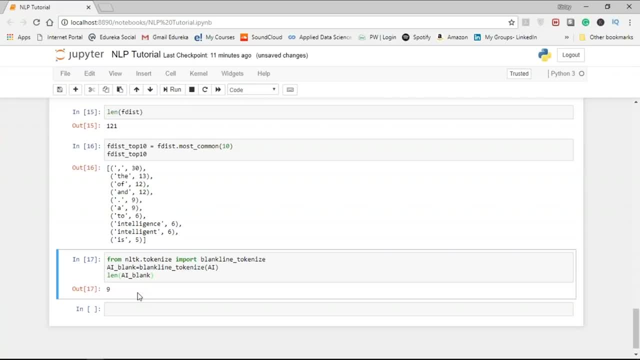 Now, what it tells us is the number of paragraphs which are separated by a new line in our given document. So suppose you want to have a look at the first paragraph, or supposedly the second paragraph, All you need to do is pass on the number and it will give you. 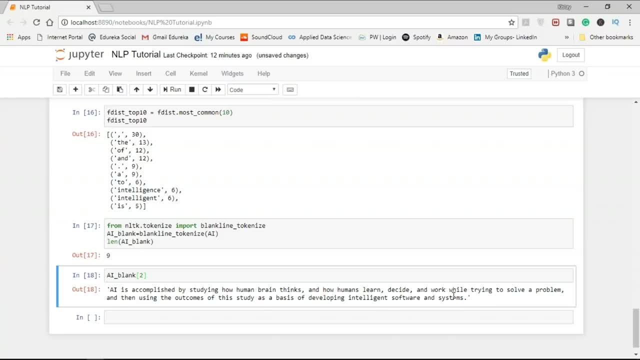 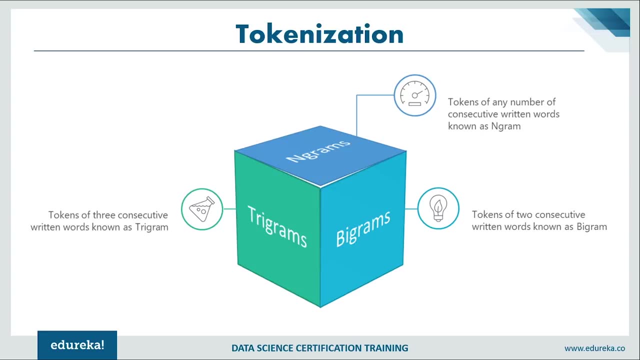 the whole paragraph, as you want, which is separated by a new line, of course. Now coming back to our tokenization part, We have bigrams, trigrams and n-grams. Now, bigrams are tokens of two consecutive written words. Similarly, trigrams refer to tokens of three consecutive. 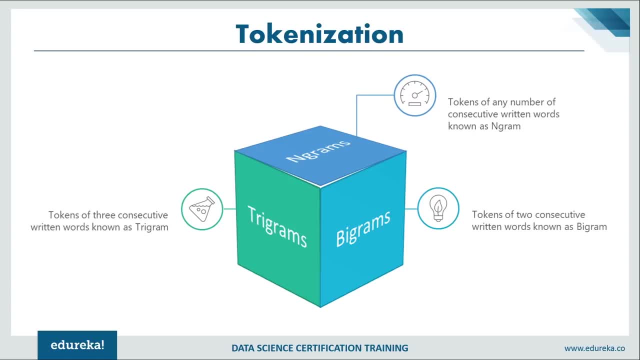 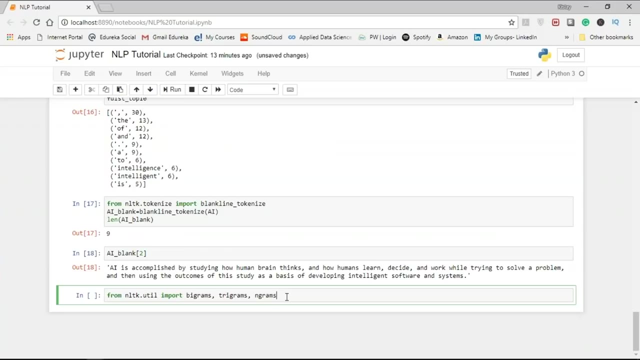 written words, and usually n-grams, is referred to as tokens of any number of consecutive written words for n numbers. So let us see how we can implement the same using NLTK libraries for bigrams, trigrams and the n-grams. So first, what we need to do is import bigrams, trigrams. 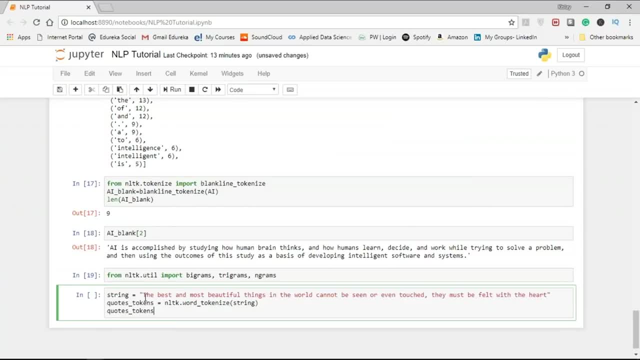 and n-grams from nltkutil. So let's take a string. the best and the most real thing in the world cannot be seen or even test. They must be filled with the heart. What a beautiful code. So let us know. first create the tokens of the string using. 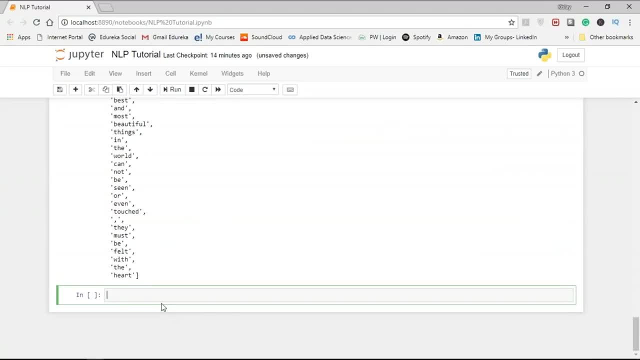 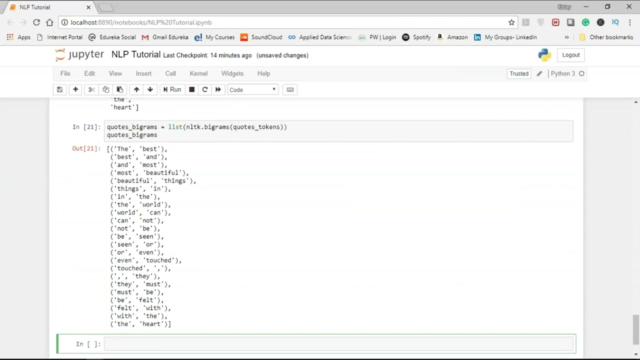 the word underscore tokenize, as I did earlier. now, to create a bigram, What we need to do is use the list function and inside that we are going to use the NLTK dot bigrams and pass on the tokens. So, as you can see, it has created a bigram of the given document. 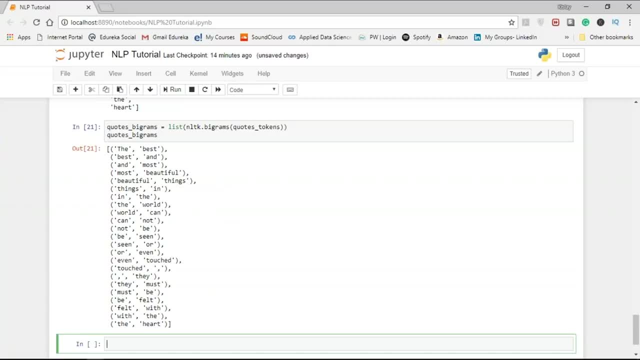 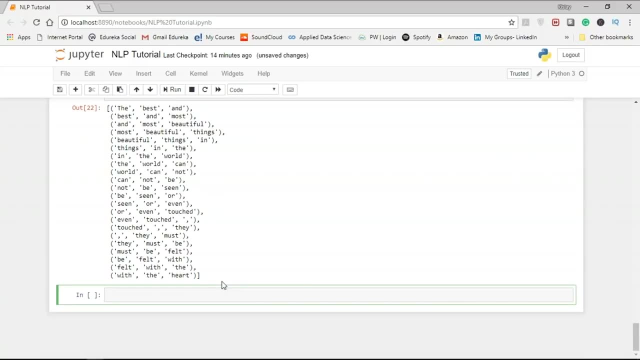 Similarly, if we create the trigrams and the n-grams, So all you need to do is change the bigrams to trigrams and it will give you the trigram list. Now let us not create an n-gram list, Okay. 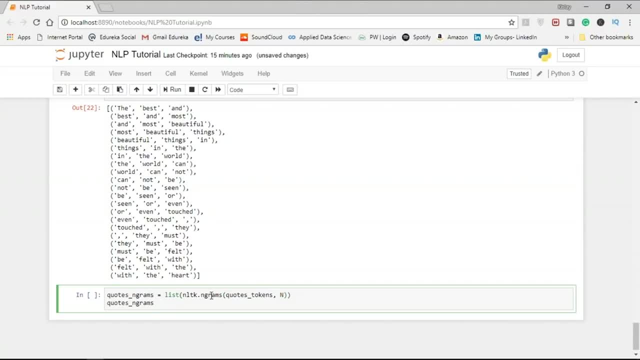 So, guys, as you can see, here we are using the same function and I'll take a dot n-grams and inside that we are passing the codes and the course token, and here, in place of n, we are going to give our number. So let's say, suppose I provide five here. 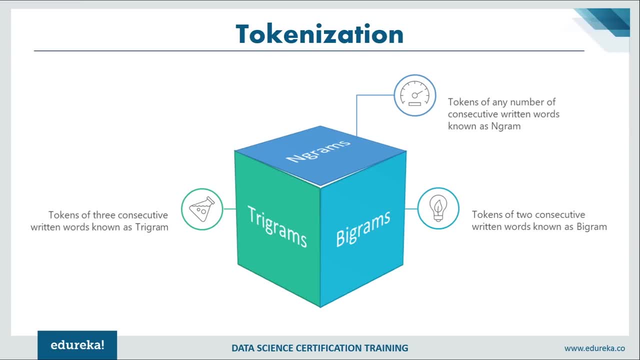 So, as you can see, it has given us an n-gram of length 5.. Now, once we have got all the words, or, as I say, the tokens, we need to make some changes to the tokens, And for that we have stemming. Now, what stemming does is normalize the words into its base. 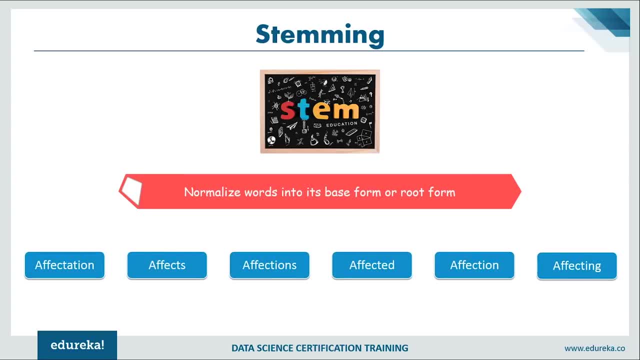 root form. So if you have a look at the words here, we have affectation, affects, affections, affected, affection and affecting. now, all of these words originated from a single root word. That is the effect. now stemming algorithm works by cutting off the end or the beginning of the word, taking into account a list. 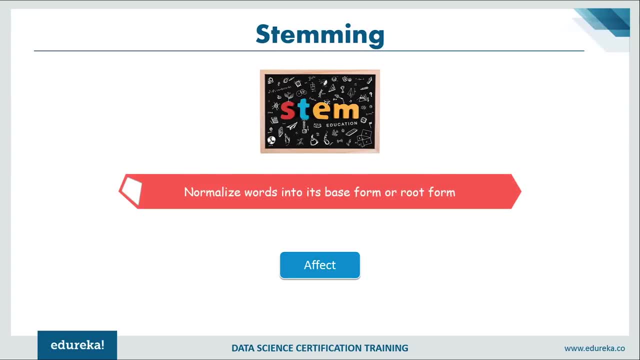 of common prefixes and suffixes that can be found in an infected world. Now, this indiscriminated cutting can be successful in some occasions, but not always, and that is why we affirm that this approach presents some limitations. Now let's see how we can implement stemming, and we'll see. 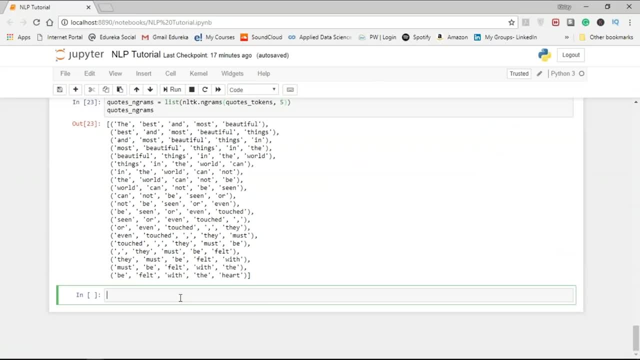 what are the limitations of stemming and how we can overcome them. Now, there are quite a few different types of stemmer, So let's start with the Porter stemmer. So for that, we are going to use from NLTK dot stem import Porter. 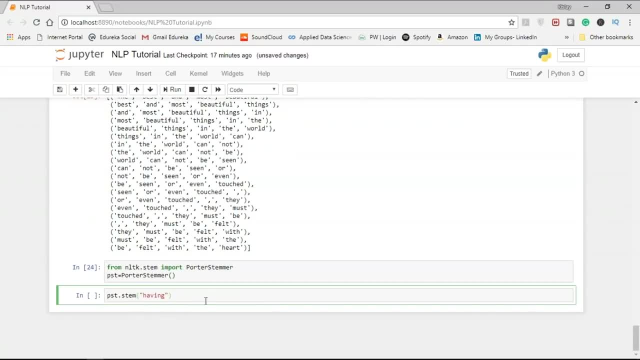 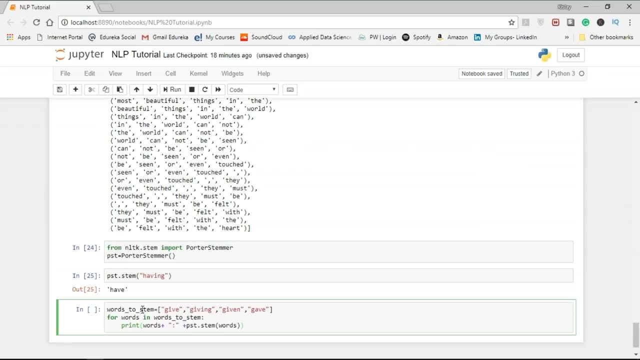 stemmer. and let's see what does this give us? The output of stemming the word having. so, as you can see, it has given us the root word. have now, similarly, if we provide a list of words such as give, giving, given and gave, and I have. 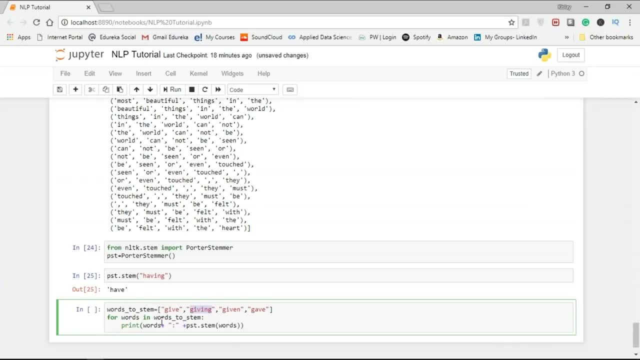 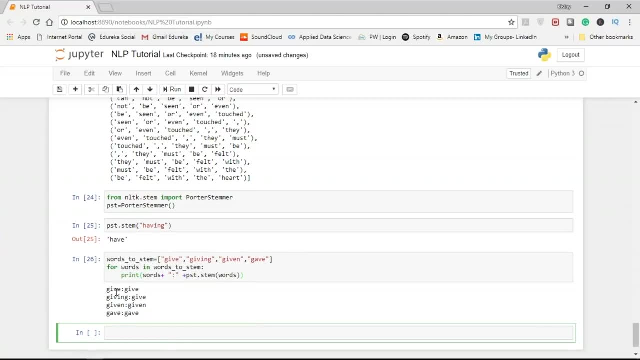 given this name of words to stem. So for words, inverse system, print words and we are using the Potter stemmer, which is the PST dot stem method, says you can see it has given us the output give, give, given and gave. so you can see the stemmer remove the only ing. 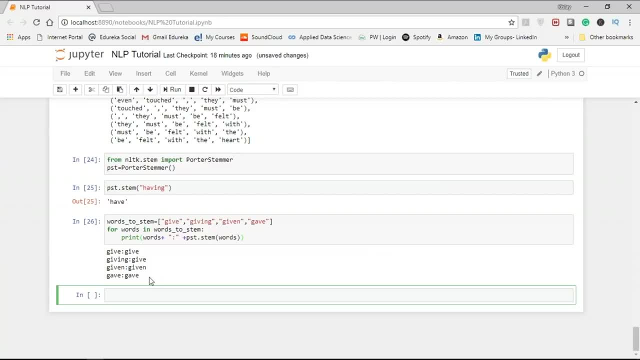 And replace it with e. now there is another stemmer, which is known as the Lancaster stemmer. So let's try to stem the same thing using the Lancaster stemmer and see what is the difference. So let's stem the same thing using the Lancaster stemmer and. 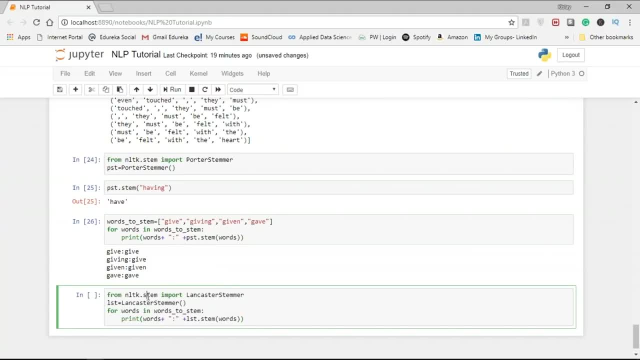 see what are the differences. we have it. So, first of all, we are going to import the Lancaster system and we are going to provide LST, which is the Lancaster system of function, and in the similar manner that we did for the Potter stemmer. 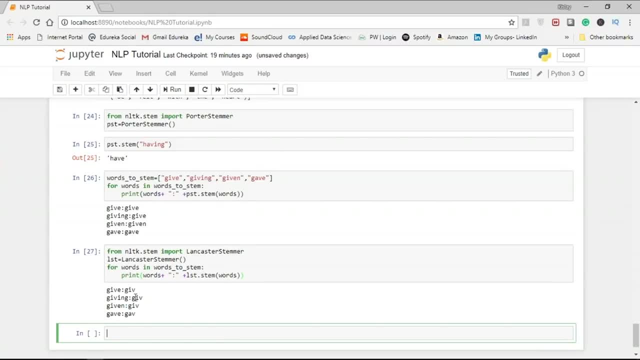 Let us execute the Lancaster system also. So, as you can see, here, the stemmer has stemmed all the words. as a result of it, You can conclude that the Lancaster stemmer is more aggressive than the Potter stemmer. Now, the use of each of the stemmers depend on the type of 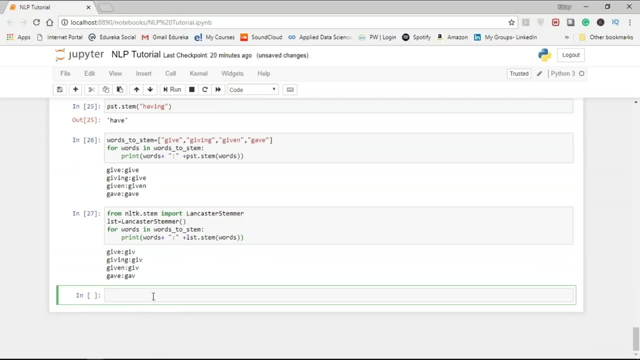 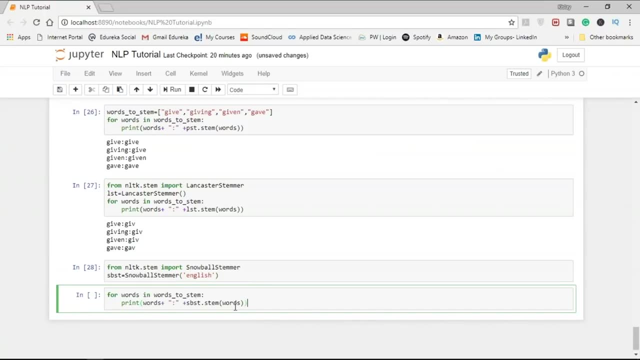 the task you want to perform. Now we have another stemmer, which is known as the Snowball stemmer. now, for Snowball stemmer, We have to provide the language which we are using. so, similarly, if we use the Snowball stemmer on the given words, as you can, 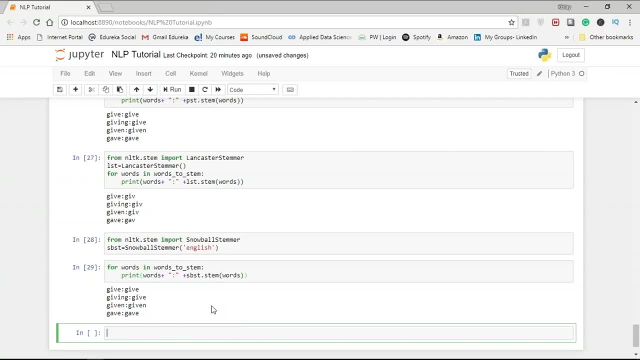 see, it has given us a different output from the previous Lancaster stemmer. So, as you can see, the output is the same as that of the Potter stemmer here, but it differs in different terms. Now, the use of each of the stemmer depends on the type of 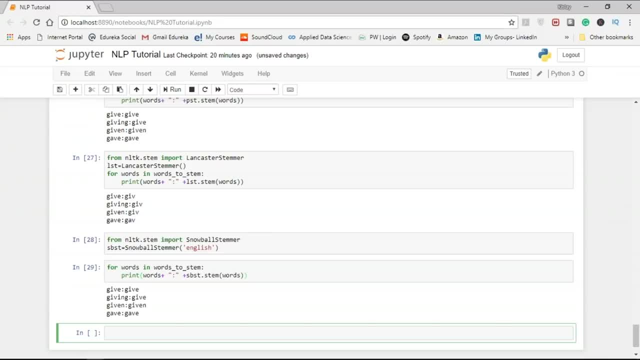 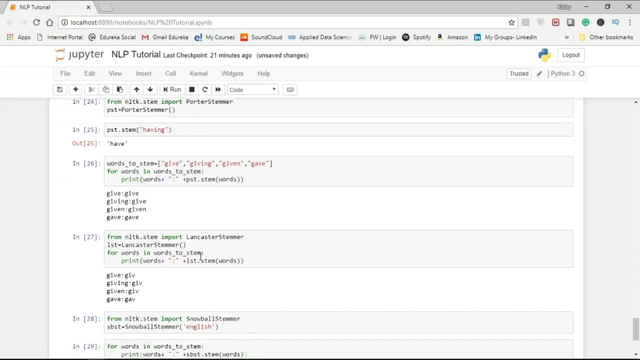 the task you want to perform. For example, if you want to check how many times the word GIV is used above, you can use the Lancaster stemmer, and for other purposes you have the Snowball stemmer and the Potter stemmer as well. 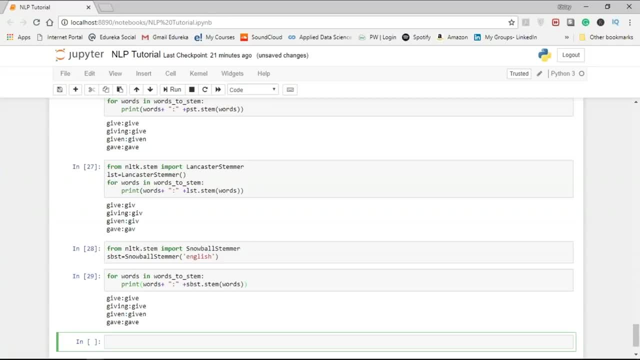 So what happens is that sometimes stemming does not work properly. It does not always Result to give us the root word. So, for example, if you take the word fish and fishes and fishing, all of that stems into fish. so lemmatization is an another concept. 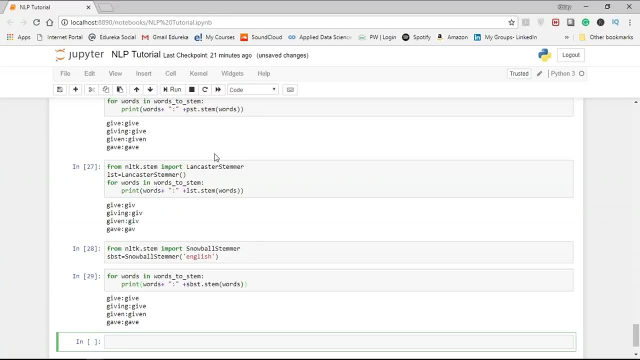 So, on one hand, where stemming usually works by cutting off the end and the beginning of the word, lemmatization takes into consideration the morphological analysis of the world. So, to do so, it is necessary to have a detailed dictionary which the algorithm can. 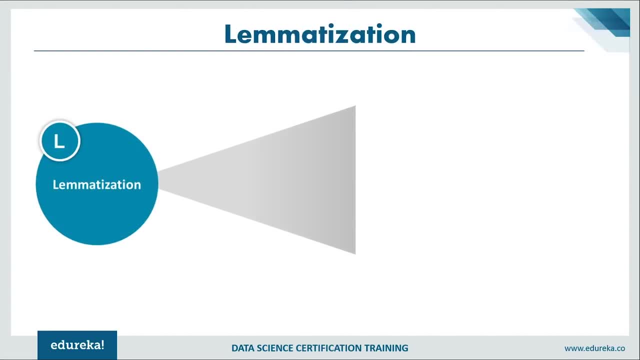 Look into to link the form back to its lemma. Now, what lemmatization does is groups together different infected forms of the word called lemma. It is somehow similar to stemming, as it maps several words into one common route. Now, one thing to keep in consideration here is the output. 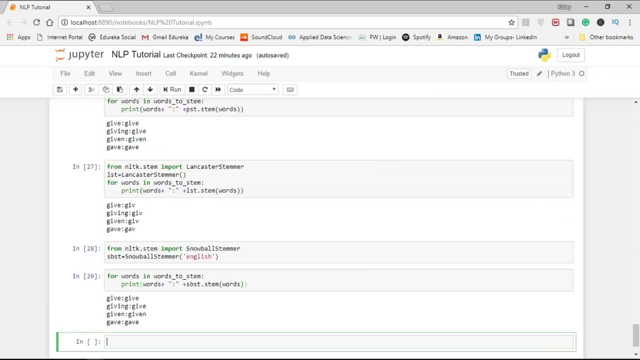 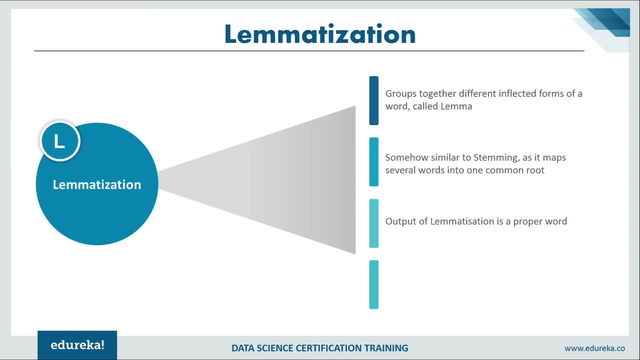 of lemmatization is a proper word. So, for example, if you look back to our output given by the Lancaster stemmer, you can see it has given us the output GIV, which is not a word. So the output of lemmatization is a proper word. 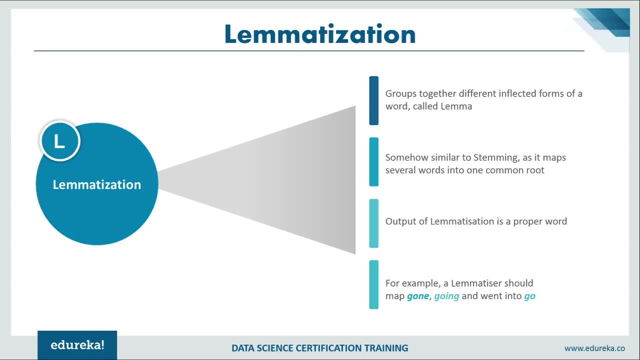 And, for example, if you take a lemmatization of gone going, it all goes into the word go. now again we can see how it works with the same example of words. Let's try lemmatization using the NLTK library. 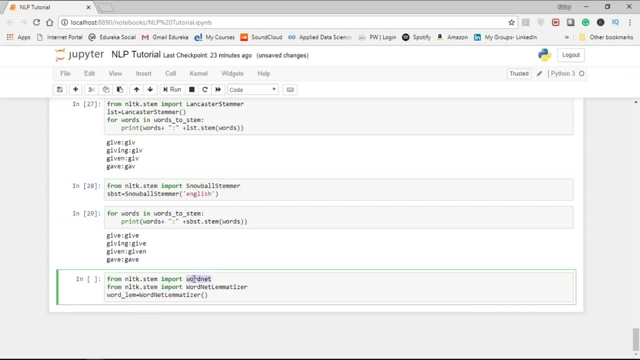 So, first of all, we are going to import the word net. as mentioned earlier, It requires a dictionary which the algorithm can look into to link back the form into its original lemma, And since the output is a perfect word, so it needs to have a 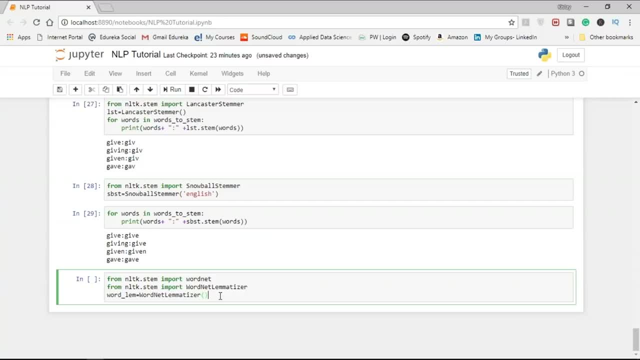 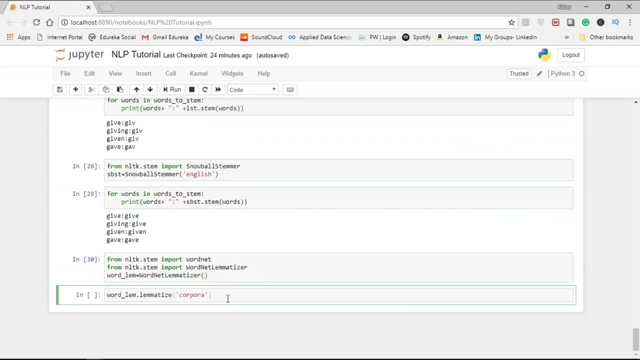 dictionary. So here we are going to import the word net dictionary and we are going to import the word net lemmatizer. So let us first take the word corporate and see what its lemma is. So what do you think, guys? What will be the output? as you can see, it has given the right. 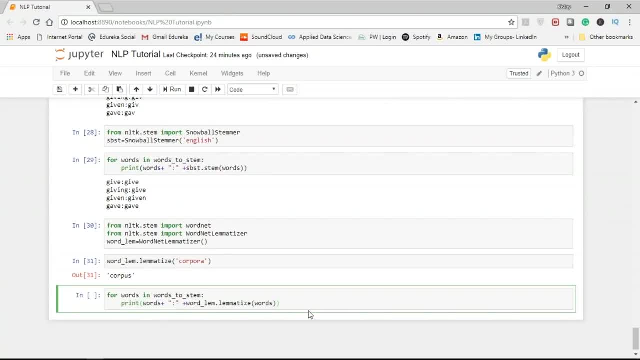 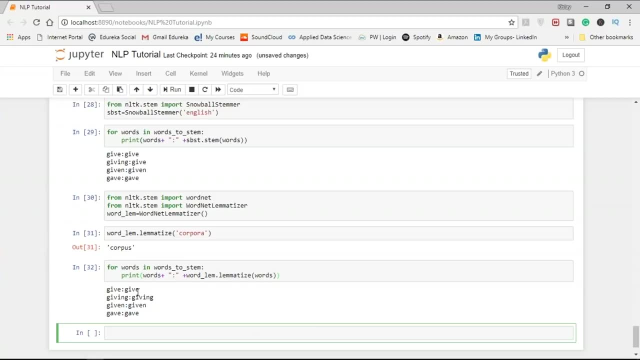 output, which is the corpus. So let's use lemmatization on the given words. So, as you can see, here the lemmatizer has kept the words as it is. This is because we haven't assigned any POS tags here. 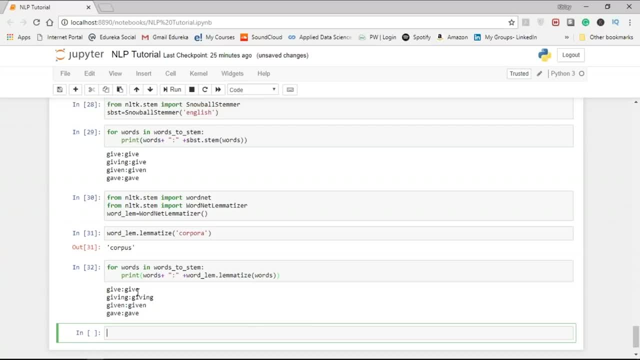 And hence it has assumed all the words as none. Now we'll learn about POS later in this video, But just to give you a hint of what POS is, POS is basically parts of speech So as to define which word is a noun, which is a pronoun. 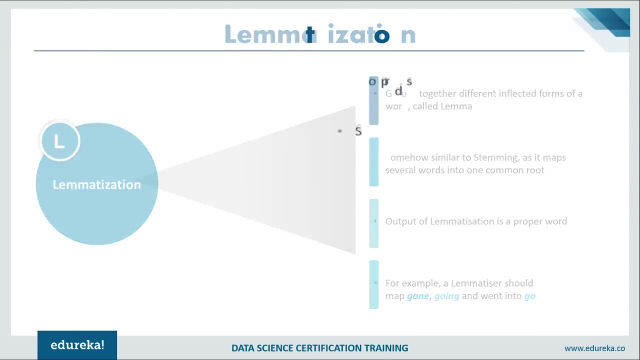 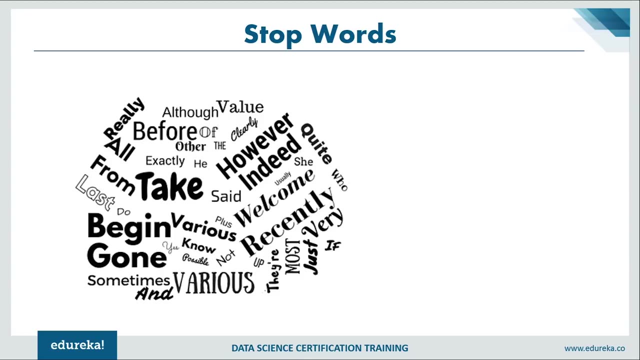 and which is a subject and much more. Now, do you know? there are several words in the English language, such as I had for begin gone No where is- which are thought of as useful in the formation of sentence, and without it the sentences won't even make sense. 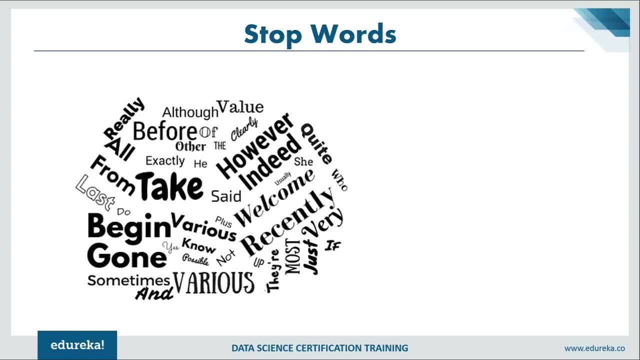 But these do not provide any help in NLP, So these lists of words are known as stop words. So you might be confused as if are they helpful or not. It is helpful in the English language, but it is not helpful in the language processing. 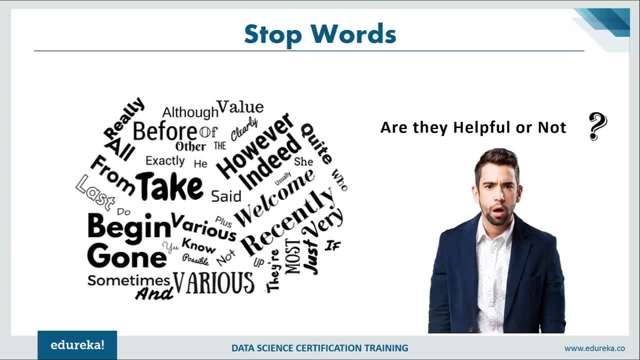 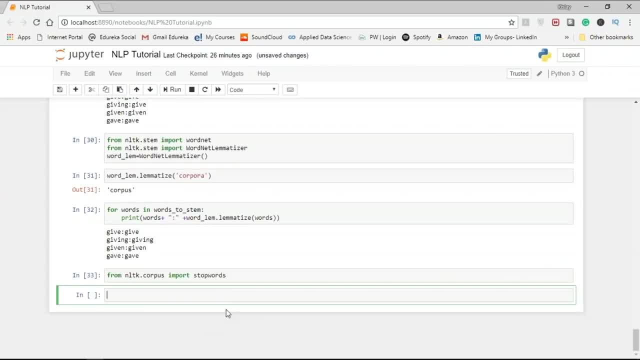 So NLTK has its own list of stop words. You can use the same by importing it from NLTK dot corpus. So once we import the stop words, we can just have a look at the different stop words which is provided by NLTK. 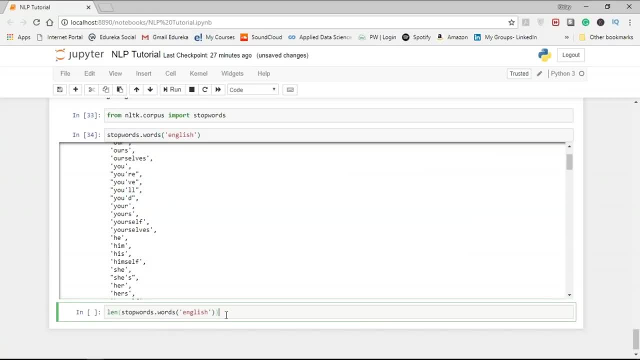 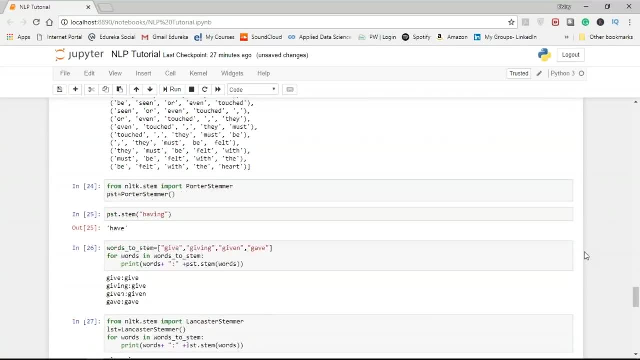 So we need to mention which language we are using. So let's have a look at the number of stop words. We have an English format, So it is 179.. So remember, guys, when we use the F dist underscore top 10 to check the top 10 tokens which have the highest number of. 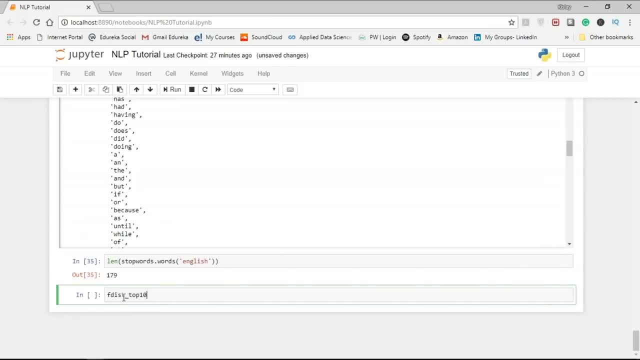 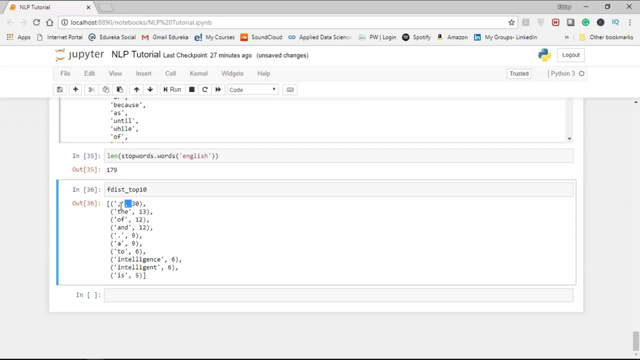 frequency. So let us take that again. So, as you can see here, apart from the word intelligence and intelligent, all of the words are usually stop words, or basically I should say that they do not match any particular word. They are like special digits and characters which do not add. 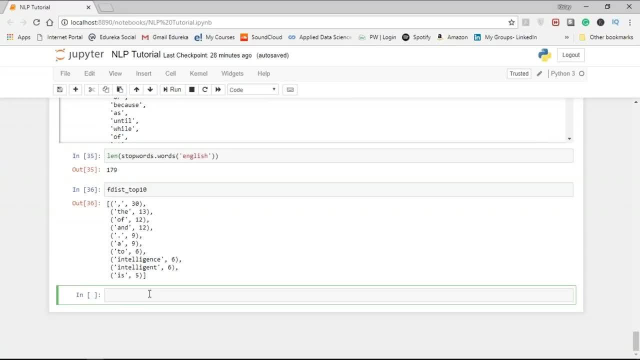 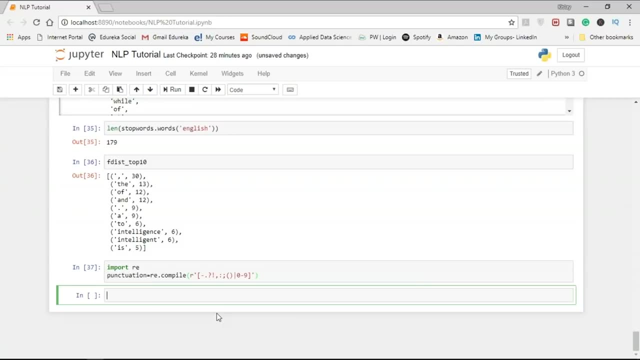 any value to the language processing and hence it can be removed. So, first of all, we will use the compile from the re module to create a string that matches any digit or the special character. Now we'll create an empty list and append. 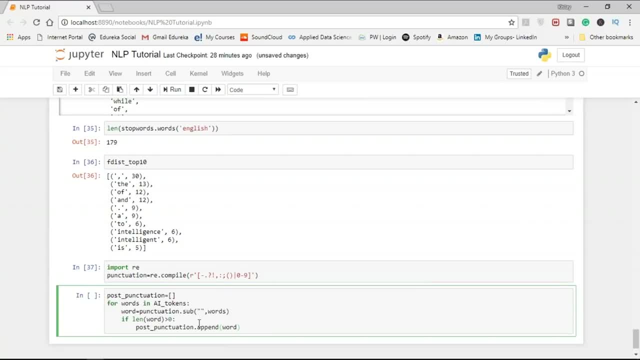 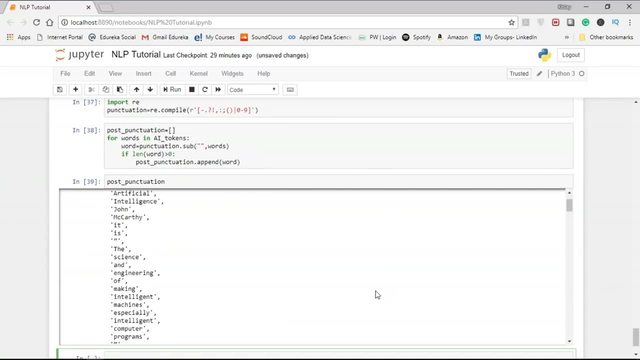 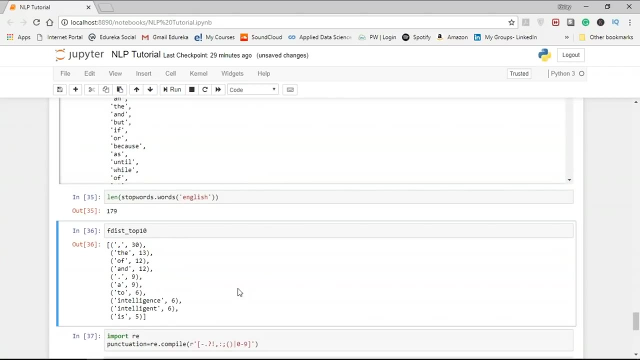 The words without any punctuation into the list. So I'm naming this as post punctuation. And if you have a look at the output of the post punctuation, so as you can see, it has removed all the various numbers and digits and the comma and the different elements. 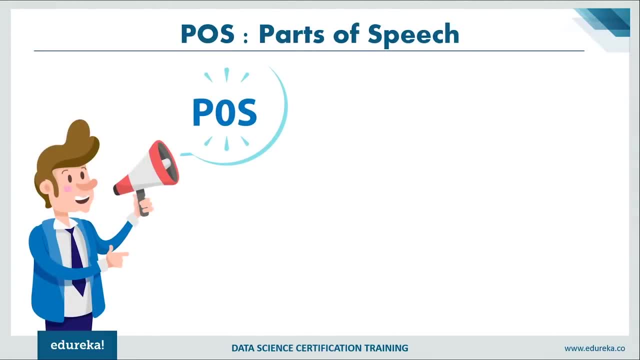 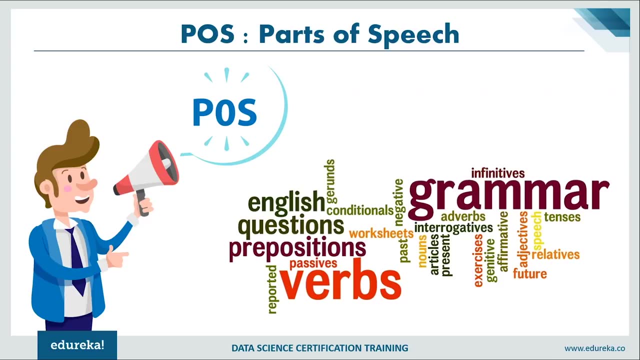 Now, when I was talking about POS, which is parts of speech, but generally speaking, the grammatical type of the word, the verb, the noun, adjective, adverb, An article. now it indicates how a word functions in meaning as well as grammatically. within the sentence a word can have: 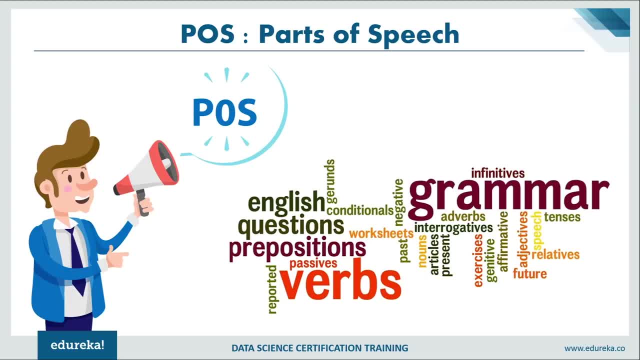 more than one parts of speech based on the context in which it is used. For example, if we take the sentence Google something on the internet, now, here, equal is used as a verb, although it is a proper noun, but these are some sort of ambiguities and 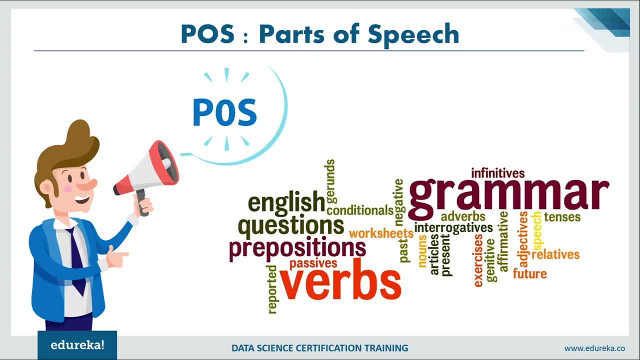 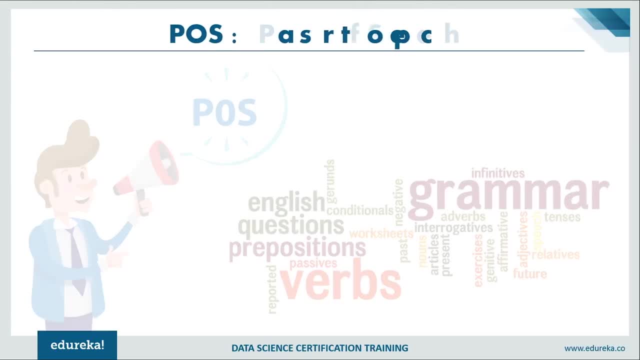 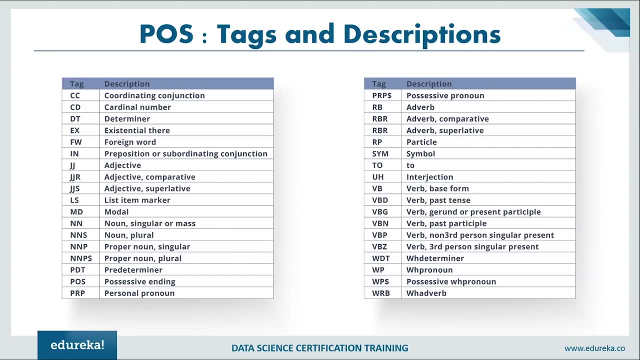 the difficulties, which makes the natural language understanding even much more harder as compared to natural language Generation, because once you understand the language, generation is pretty easy. So POS tax are usually used to describe whether the word is a noun, an adjective, a pronoun, a proper noun, singular ruler. 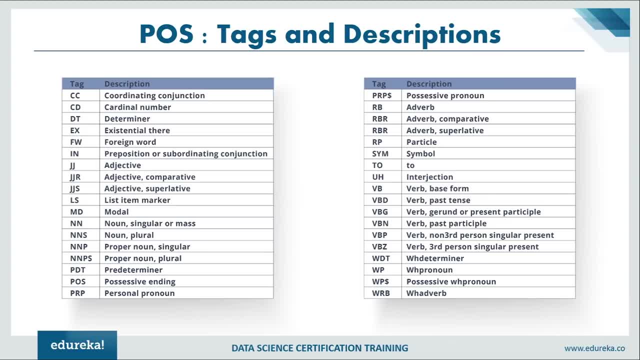 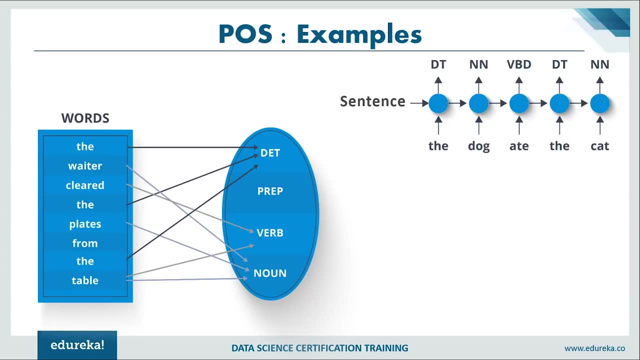 verb, Is it a symbol? Is it an adverb? So, as you can see, here we have so many tags and descriptions for the different kinds of words, all the way ranging from coordinating conjunction to what work wrp. Now let's take an example of these two sentences. 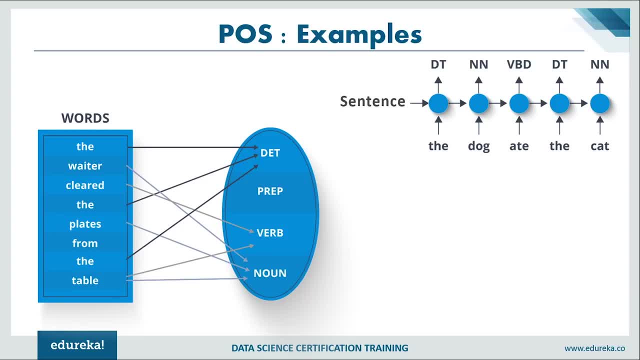 So the first sentence is: the waiter cleared the plates from the table. So, as you can see from the starting, if we use the word take into consideration, though it is a determiner now, waiter is a noun, cleared is a verb, though is again determiner- the plates. 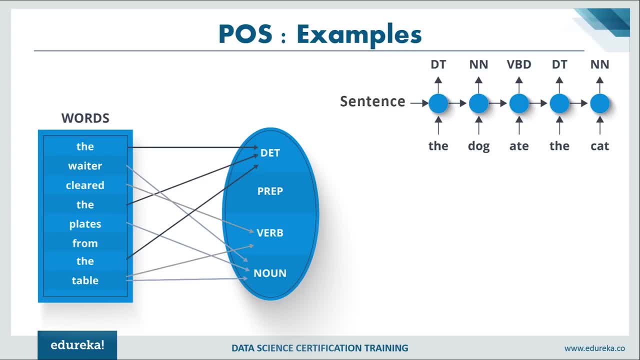 are noun from is not defined. here, though, is again the determiner, and the table is again a noun. now again, if we take into consideration the sentence, the dog ate the cat. Similarly does the determiner dog. noun 8 is the world, and again it's the same to the minor and the noun. 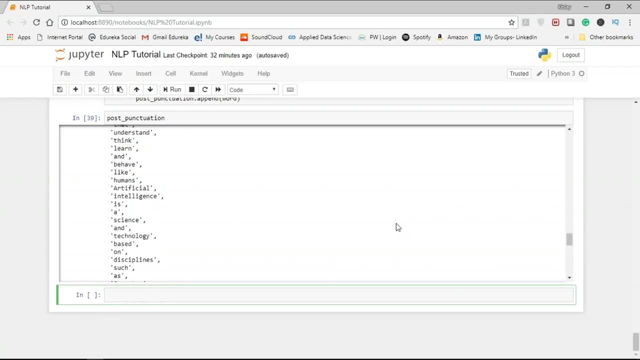 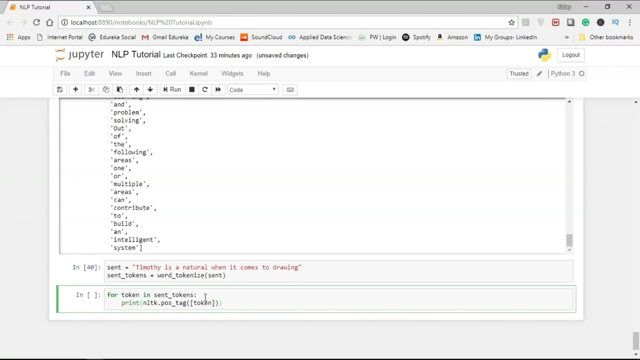 So let's see how we can implement POS tax and do the tagging using the NLTK library. So let us take a sentence. Timothy is a natural when it comes to drawing. first of all, we'll tokenize it using the word underscore tokenize, And then we are going to use the POS underscore tag on all. 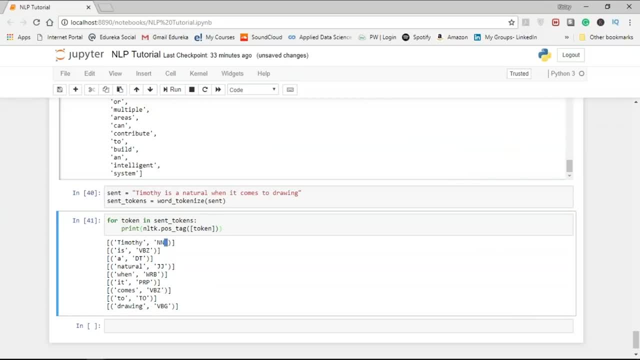 of these tokens. So, as you can see, it has. Define Timothy as a noun, is as a verb, as a determiner, natural as an adjective, when as a WRB adjective, and it as a preposition. it comes as a verb to and drawing as a verb as well. 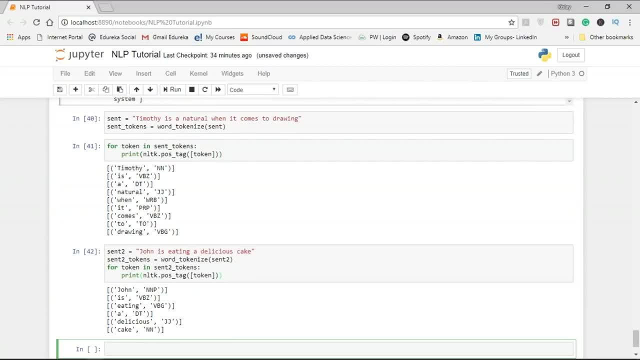 Now let's take another example- that John is eating a delicious cake. So, as you can see here, the tagger has tagged both the is and eating as well, because it has considered is eating as a single term. Now, this is one of the. 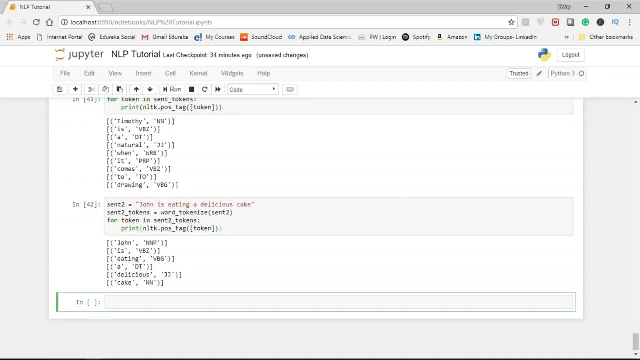 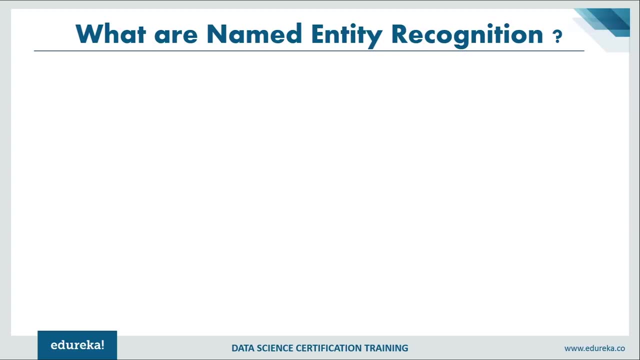 Shortcomings of the POS taggers when it comes to tying the words. Now, another concept in natural language processing is NER, which is known as named entity recognition. So the process of detecting the named entities, such as a movie, a monetary value, be it an organization, a location, quantities. 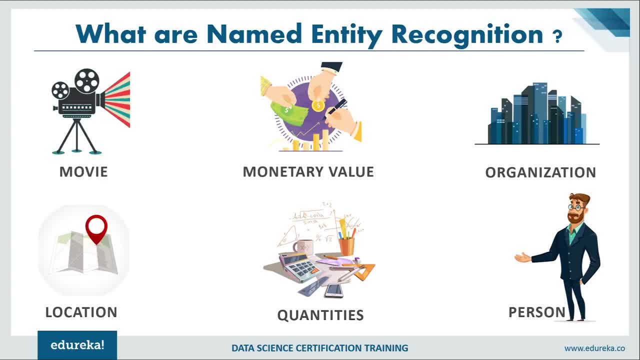 and a person from a text is known as named entities recognition. Now, there are three phases of NER, which is first is the noun phrase identification. Now this step deals with extracting all the noun phrases from a text using dependency, passing and parts of speech. 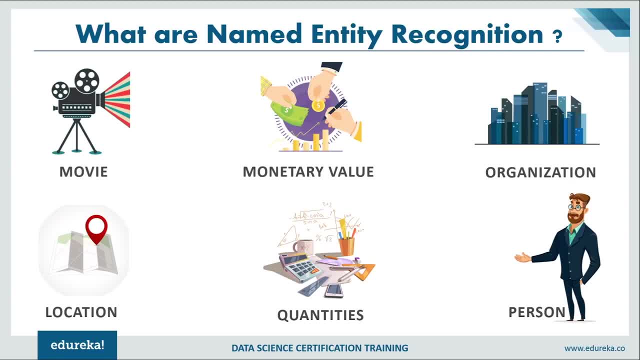 tagging, which is the POS tag Now. Secondly, we have to phrase classification. Now, this is the classification step, in which all the extracted nouns and phrases are classified into respective categories, such as location names and much more. now, apart from this, one can curate the lookup tables and dictionaries by combining: 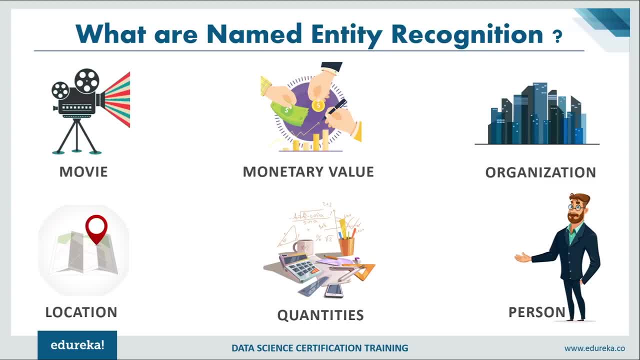 information from the different sources. And finally, we have the entity disambiguation. Now, sometimes it is possible that the entities are misclassified, as creating a validation layer on top of the result is very useful. The use of knowledge graphs can be exploited for this purpose. 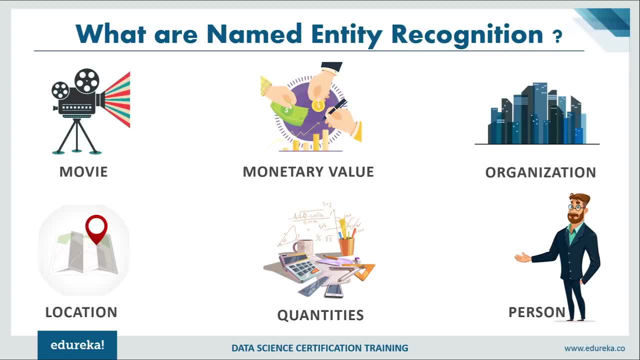 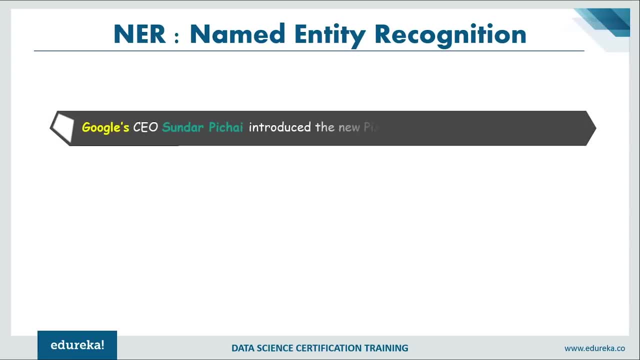 Now the popular knowledge crafts are the Google knowledge craft, the IBM Watson and also Wikipedia. So if we have a look at a certain example- suppose this is the sentence- the Google CEO, Sundar Pichai, introduced A new pixel at Minnesota Roy Center event. 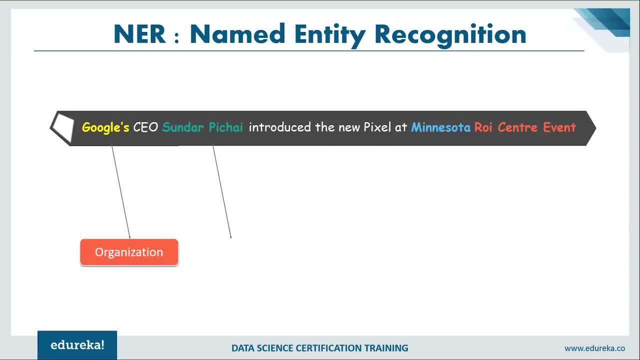 So, as you can see, Google is an organization, Sundar Pichai is a person, Minnesota is a location and Roy Center event is also an organization. This is an additional layer on top of the POS tagging so as to clarify and give us more depth into what the sentence is. 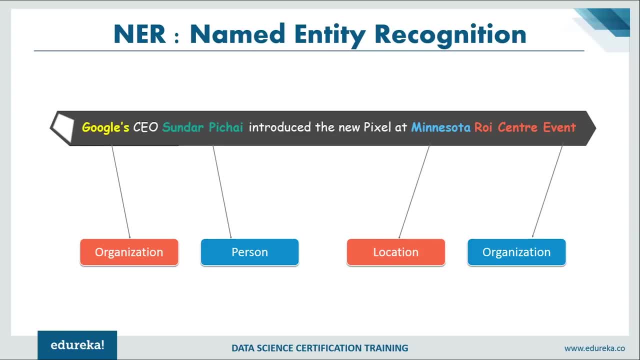 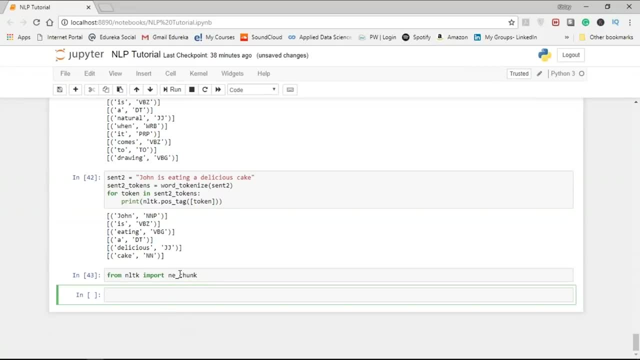 about and what the sentence is conveying us. So for using any are in python, you need to import the any underscore chunk from the NLT K module in python. So once we have imported any underscore chunk, now let us take this sentence into consideration, which is the US. 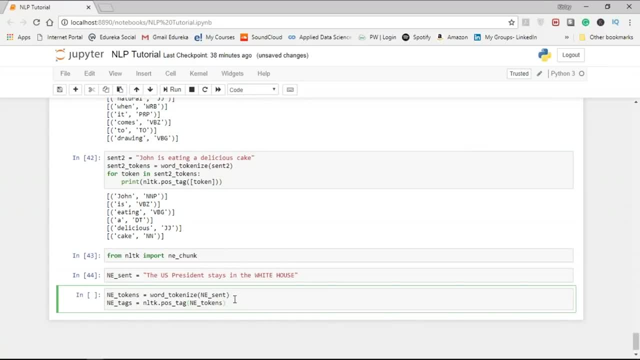 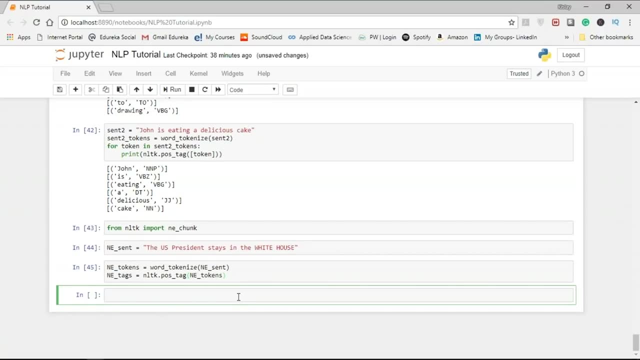 president stays in the White House. Now again, what we need to do is tokenize this sentence and after tokenizing, what we need to do is add the POS tags so that it will be easier for us to conclude the any hours. So we are passing the any underscore tags into any underscore. 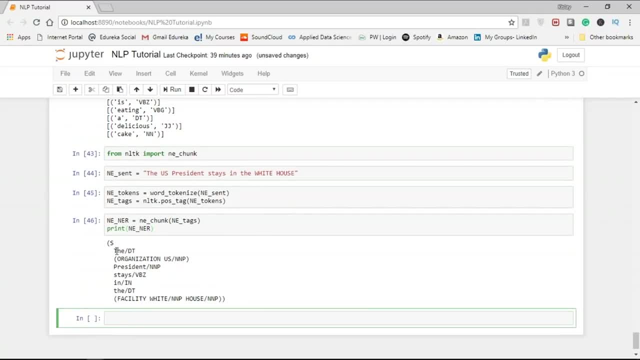 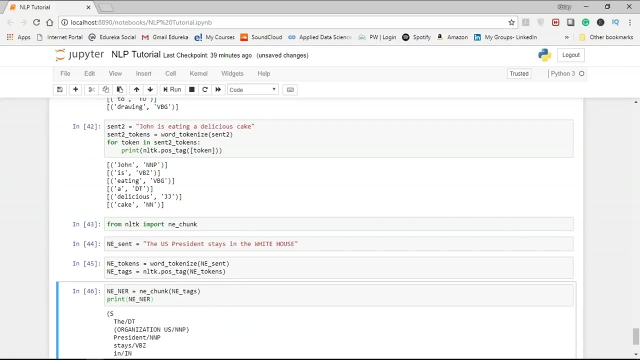 chunks function. Let's see What's the output So you can see it has given the as a determiner, It has given us as an organization and White House is club together as a single entity and just considered as a facility. So, as you can see, adding a layer of dictionary and then adding 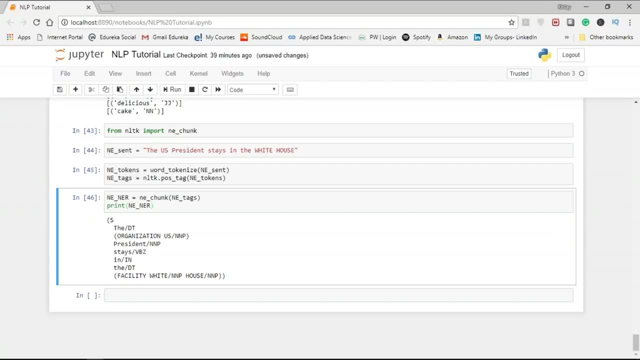 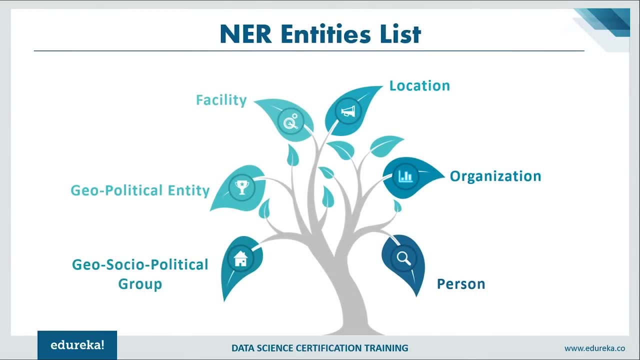 the tags and then creating the name entity recognition makes the understanding of language so much more easier. Now, as you can see in the NER entity list, we have geosocial political group. in geopolitical entity We have facility, location, organization and person says you: 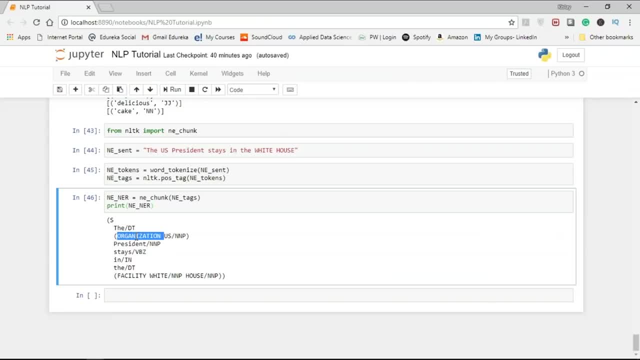 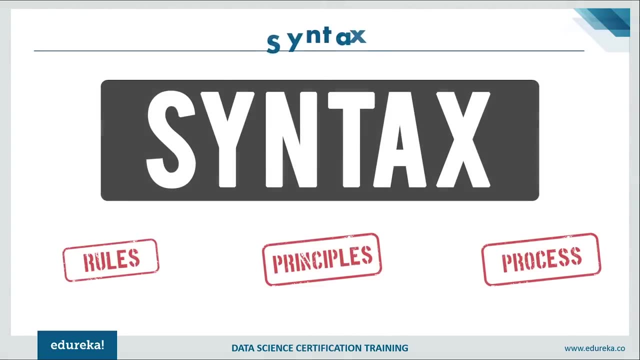 saw just from the previous example. as you can see, if we have given organization, we have facility. now an important thing to consider in NLP is also the syntax. now, in a linguistics, syntax is the set of rules, principles and the processes that govern the structure of a sentence in a given language. the 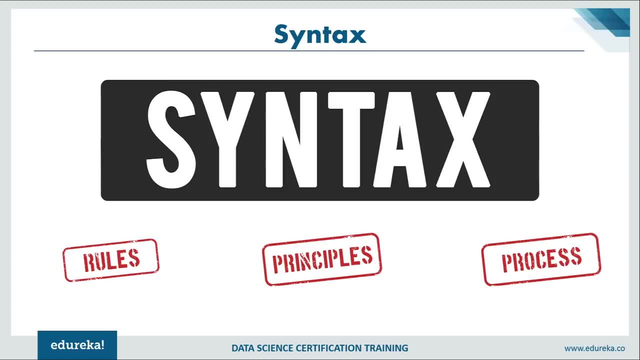 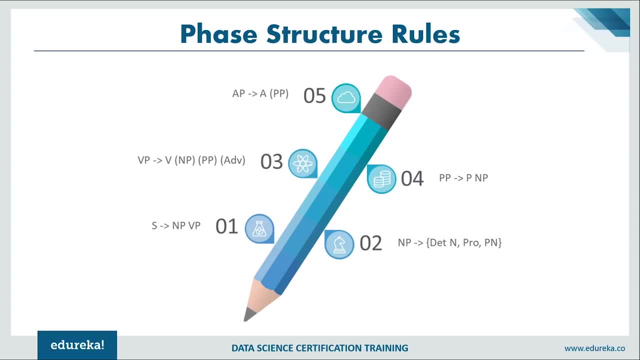 term syntax Is also used to refer to the study of such principles and processes. So we have a certain rules as to what part of sentence should come up at what position. now, with these rules, we create a syntax tree whenever there is a sentence as an input. 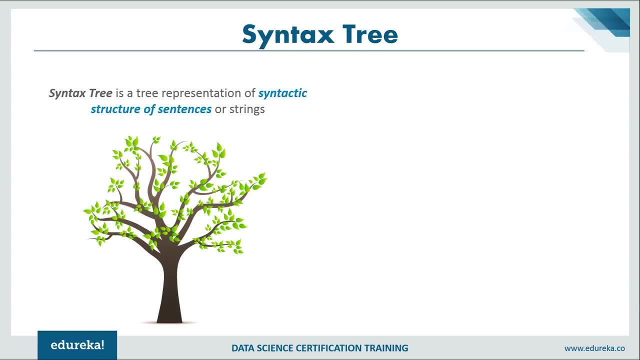 So syntax tree in layman terms is basically a tree representation of the syntactic structure of sentences or strings. Now it is a way of representing the syntax of a programming language as a hierarchical tree, like structure, And this structure is used for generating symbol tables for 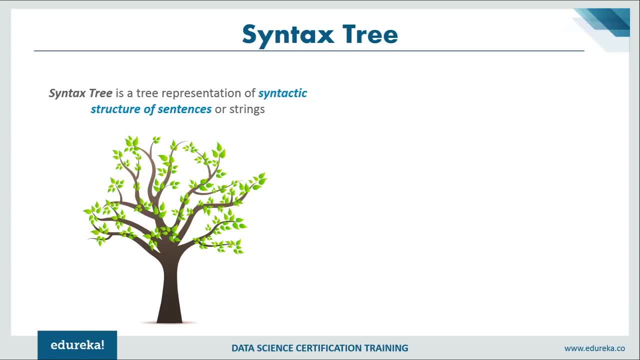 compilers and later code generation. the tree represents all the constructs in the language and their subsequent rules. now consider the statement the cat sat on a mat. So, as you can see, this is how a syntax tree looks like. we have a sentence, We have the noun phrase, the preposition phrase and again the 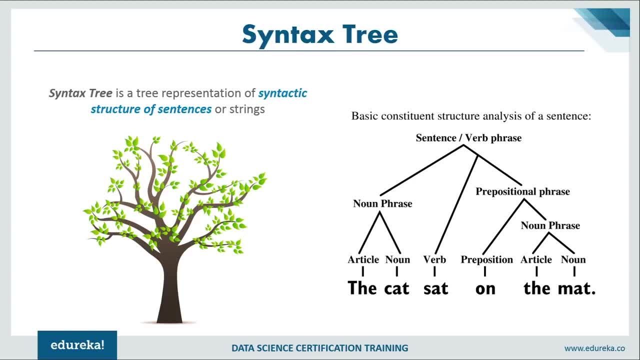 noun phrase is divided into article and noun, then we have the verb, which is sat, again We have the preposition, which is on and again, And finally we have the noun phrase, which consists of article and the noun. now, in order to render syntax trees in your 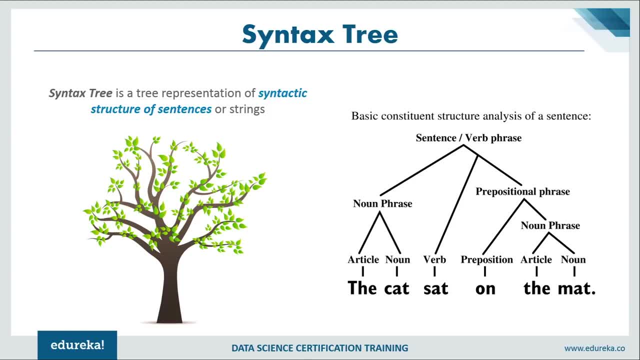 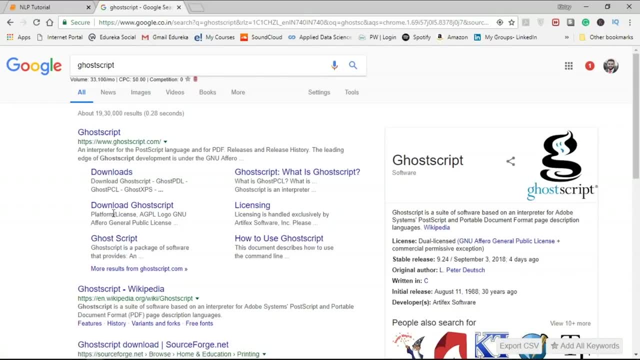 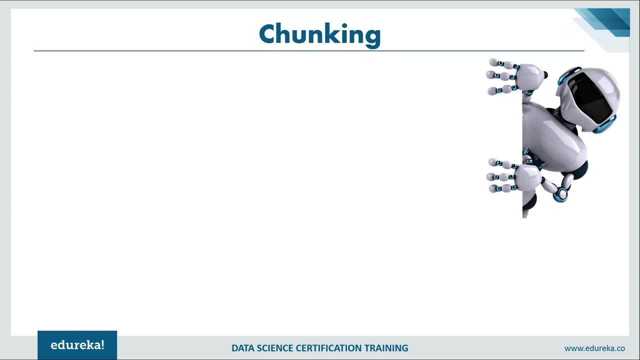 notebook. you need to install ghostrips, which is a rendering engine, So you can download ghostrips from this downloads page and not go much into the details of that. Now let us discuss an important concept with respect to analyzing the sentence structure, which is chunking, now chunking. 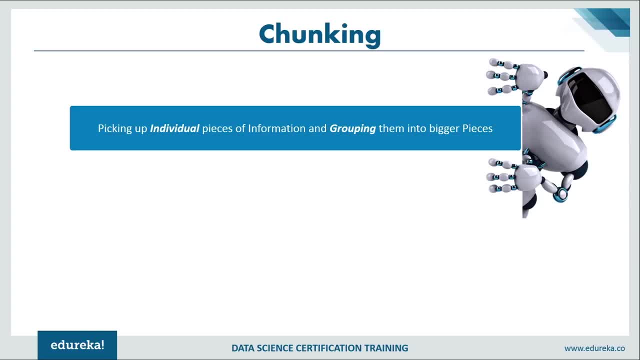 Basically means picking up individual pieces of information and grouping them into bigger pieces. So, as we saw earlier, that we have a sentence and we divided it into different tokens. that was tokenization, and this is sort of like the opposite part, or we should say the opposite. 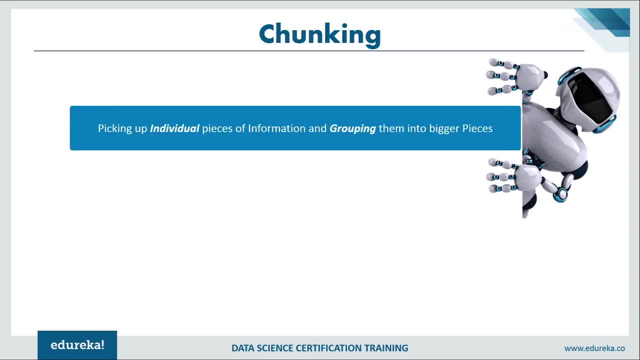 of what we can do as tokenization. a little bit of changes to that tokenization part. We'll see what are the different changes now. the bigger pieces are usually known as chunks here. now, in the context of NLP, Chunking means grouping of words or the tokens into chunks. 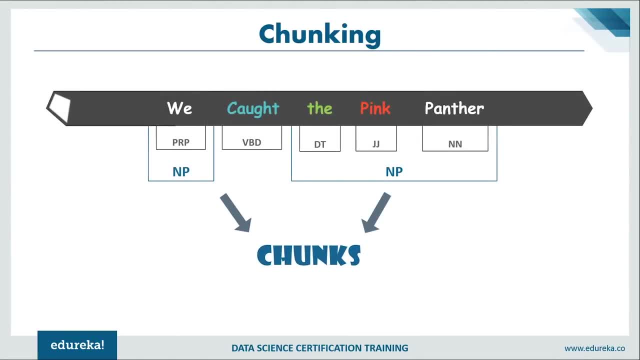 Now let's have a look at the example of chunking here. So let's consider the statement: we caught the pink Panther. So, as you can see here, the pink, which is an adjective, Panther, which is a noun, and the, which is the determiner, are chunked. 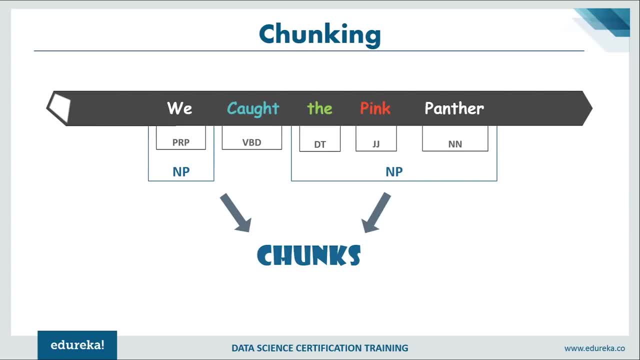 together into a noun phrase, But this also helps in determining and the processing of the language. So suppose if someone is asking Whom did we caught this morning, So the regular response to this question would be: we caught the pink Panther. now the question is asking: who so the pink? 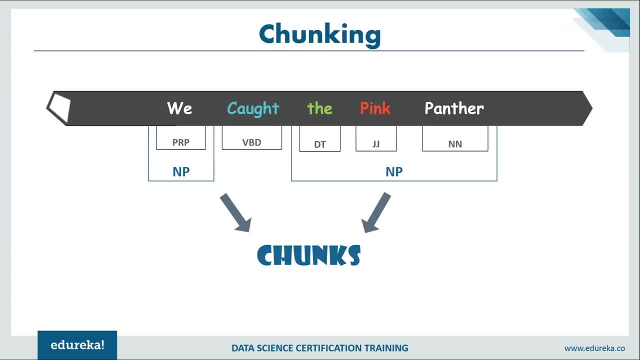 Panther becomes a noun phrase, basically. So this is something. what the chunking does is that it understands the language, and when it has understood, what it does is basically picks up the individual pieces of information and groups them into chunks so that it will be easier for us to process that data. 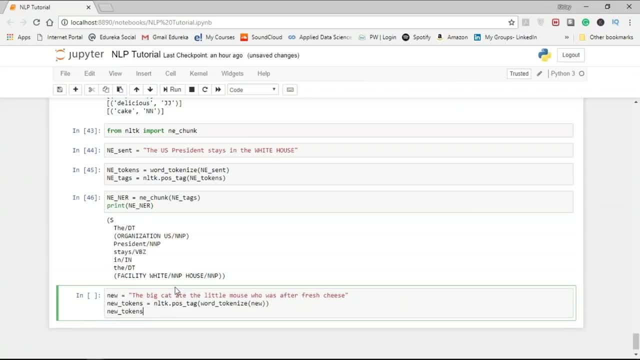 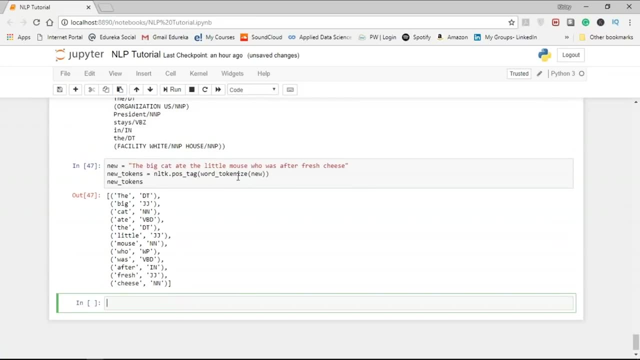 So let's take a new sentence: The big cat ate Little Mouse, who was after the fresh cheese. So let's tokenize it and add the POS tags also. So, as you can see, just under one line, or I should say in one command, I have tokenized it and I've added the POS tags also. 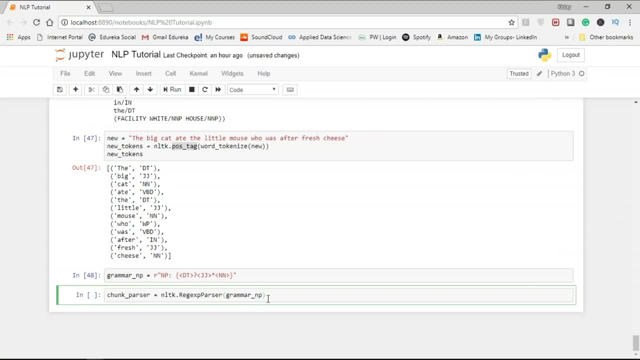 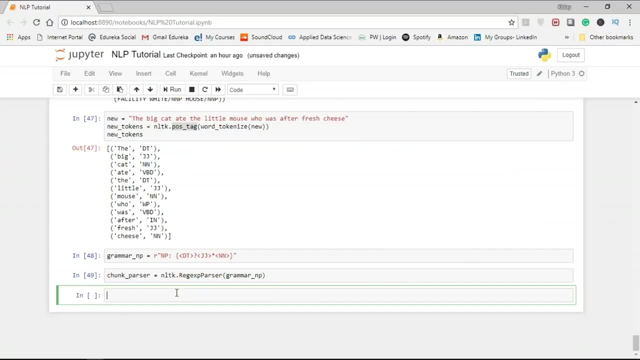 So let's define the grammar here. So next, what we are going to do is create a regular expression parser for the grammar NP, which is the grammar which we have provided, and then we'll create the chunk, The score result, and will pass this whole sentence, or I should. 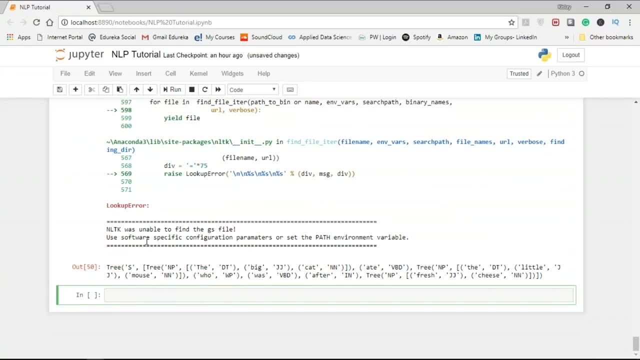 say the tokens into the chunks. There was a slight error, as NLT was unable to file the GS file, But, as you can see, here we have a tree in which the NP is the big cat. The big cat is a noun phrase. 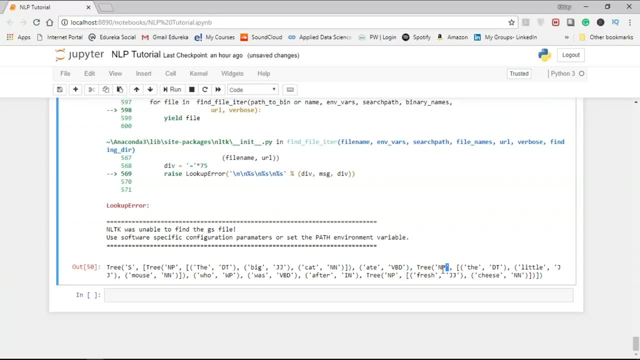 It is a verb tree. Then again we have the noun phrase, which is the little mouse, who is a word phrase, was is a verb after is in, and again we have the noun phrase, The fresh cheese. So you can see, here, although we do not have a particular tree, 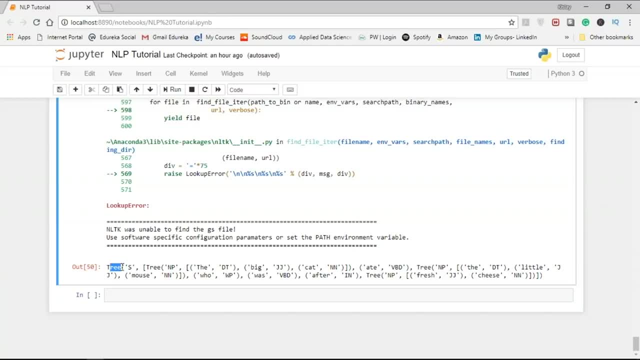 like structure. we can see that from the outer. We can see we have a tree starting from the start is here and the end is here and you can see it starts with the noun phrase The big cat, not the big cat, As I mentioned earlier in our previous example. similarly to: 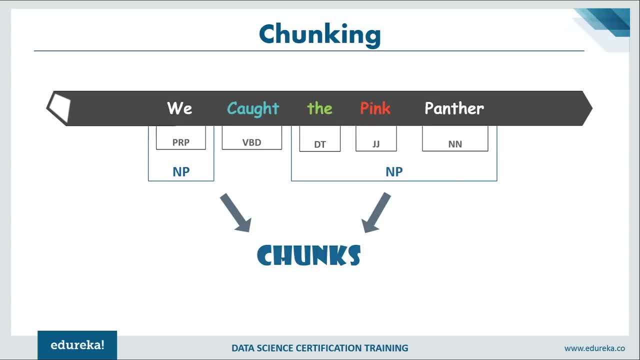 the beeping Panther. It has been taken into consideration as a noun phrase, which is basically a chunk, and it has created different chunks in the given sentence I should say. So this is it, guys. I hope you got an idea of what the different parts of NLP is. 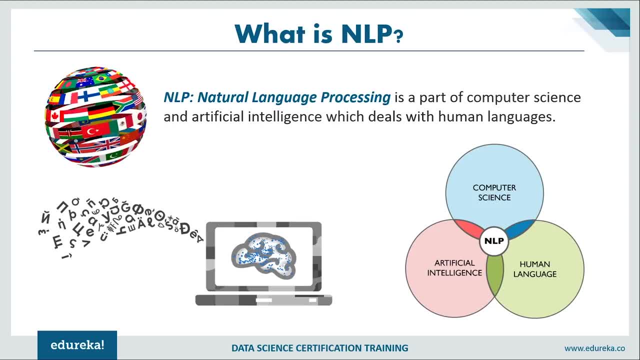 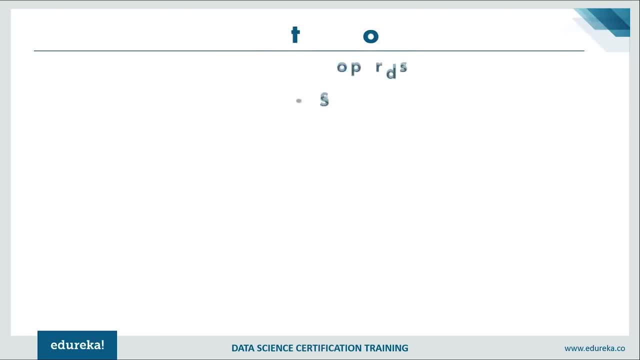 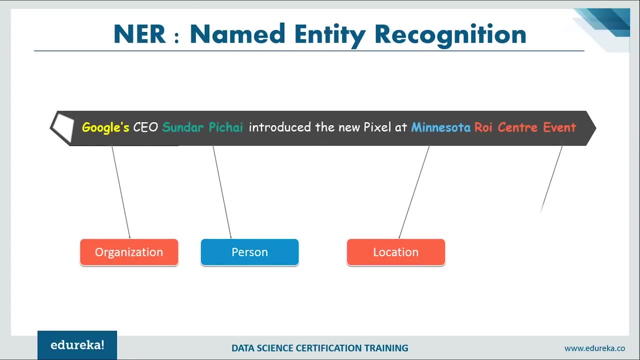 What is NLP, How it is used, the different elements of NLP, such as starting from tokenization, stop words, stemming, limit, ization. again We have the stop words, part of speech, POS tags- any are named, entity recognition and after any are. we had the syntax we created. 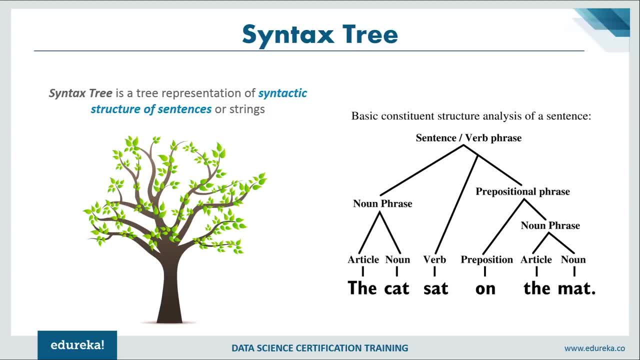 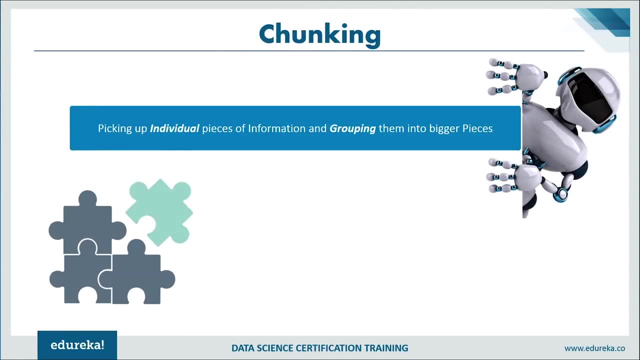 a syntax tree to know how exactly the sentence is arranged and how it uses the dictionary, the POS tags and the tokenization to create a particular tree so as to form a meaning out of that sentence. And finally, we are using chunking as to chunk together the 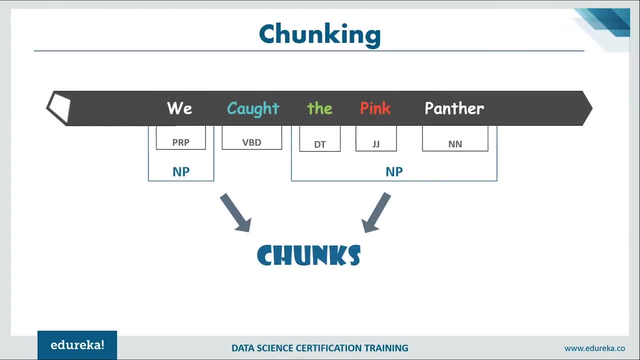 small tokens into meaningful words. So, guys, I hope you like this session and I'm sure you guys will start implementing these procedures on the given text, using the NLT canary. and let me tell you one thing, guys: The NLT canary is filled with lots and lots of text, data and 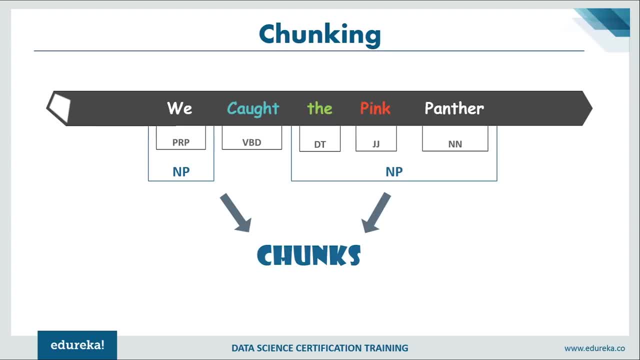 lots and lots of example. This is just the beginning of it and you can dig deeper into NLP and go into topics like context, free grammar and much more, which is already there in the NLTK package and is very useful when it comes to natural language processing. Thank you.